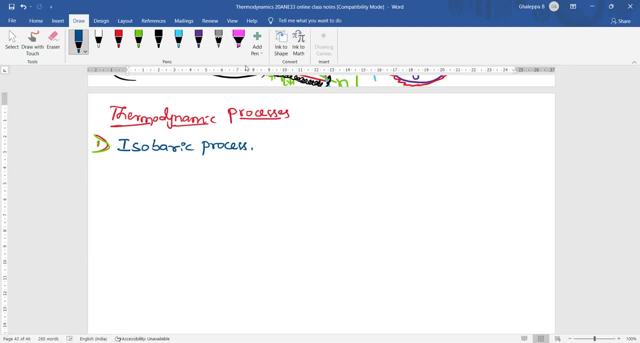 Pressure, Pressure, sir, Pressure, very good, Pressure is equal to constant. What is second process, Isobaric? Isobaric process, Which property remains constant: Volume: Volume. change in volume during the process is constant. Change in the volume is zero, actually, Change in. 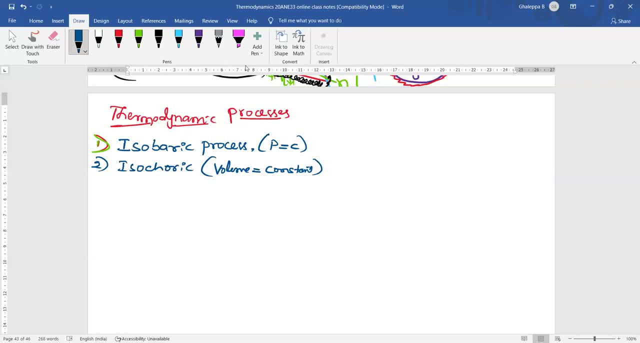 the volume is zero. Okay, volume at first point and second. Second point is the same. What is third? Thermal, Iso thermal. Okay, So which property remains constant during the process? Temperature. Temperature is equal to constant, Just you. 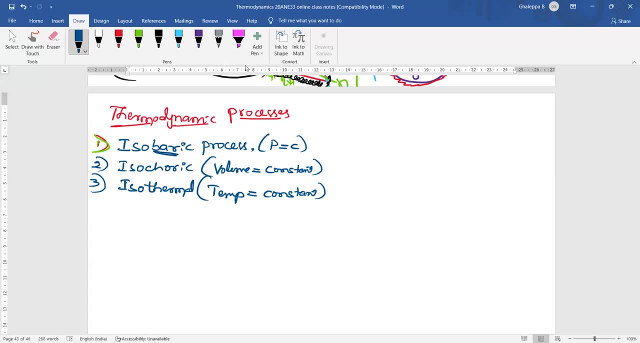 remember the hint? okay, Bar is a unit of pressure, So pressure is constant. Coric is related to volume. Volume is constant. T for temperature. Temperature is equal to constant One. Okay, here there is no property remains constant. No, But what will be the constant? 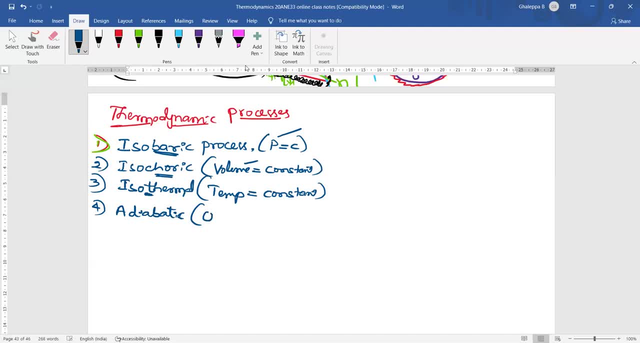 No exchange of heat. There is no exchange of heat. Yes, sir, Heat exchange is zero. Heat exchange where Between system and surrounding, Okay, Heat exchange is zero. So between device or machine, From the machine to the surrounding. 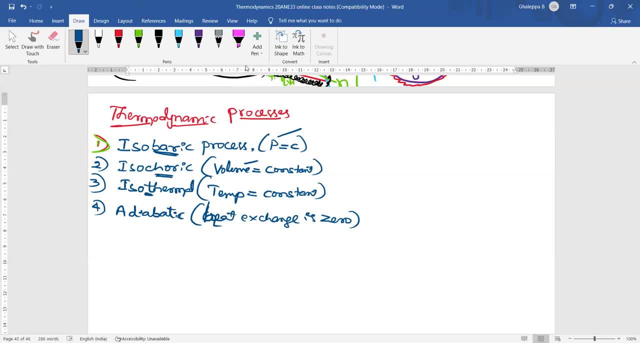 No heat exchange Heat exchange. Or from surrounding to machine: no heat exchange. Last one is polytropic: Polytropic process. So this class is very important, my dear students, to solve numericals. Okay, I will be explaining the equations as well as some important points. 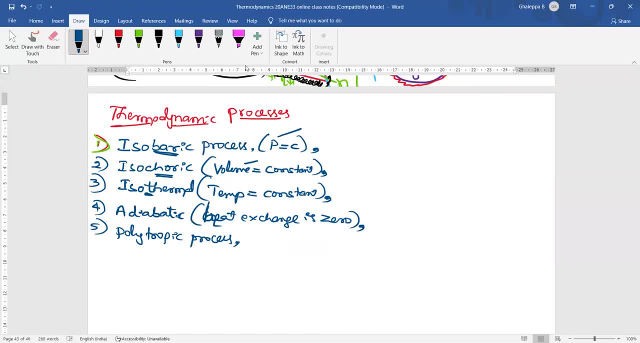 related to thermodynamic numericals. Okay, First point, what I will explain in all these cases: okay, PV diagram: how to draw PV diagram for this. How to draw a PV diagram for this. P means for pressure. it should be straight line. Okay, V means volume. Okay, V means straight line Pressure versus. 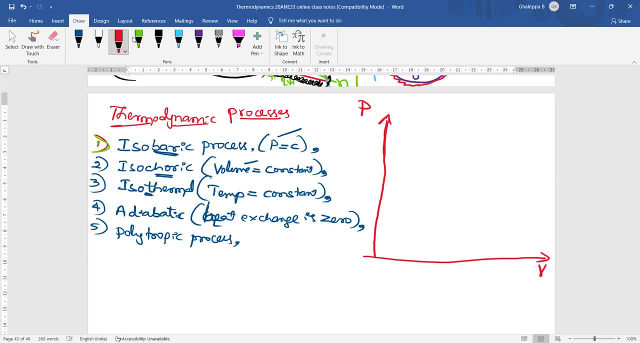 P means volume, Okay, V means volume, Okay, Mah, congratulations, no problem, Volume Thanks. like and say: how can I express vem per moment time with solENN, interesting slide, Okay. So then one more diagram will come, that is. 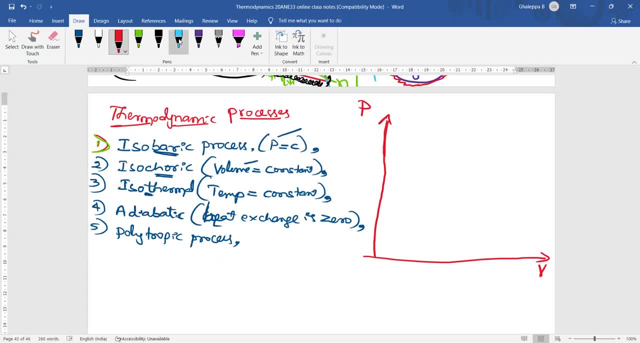 entropy, okay, so i need to tell one more point here. when it comes to entropy, dear students, look at the point number four. point number four is adiabatic, the reversible adiabatic. okay, i'm adding one more word. reversible adiabatic process is also called isentropic process. 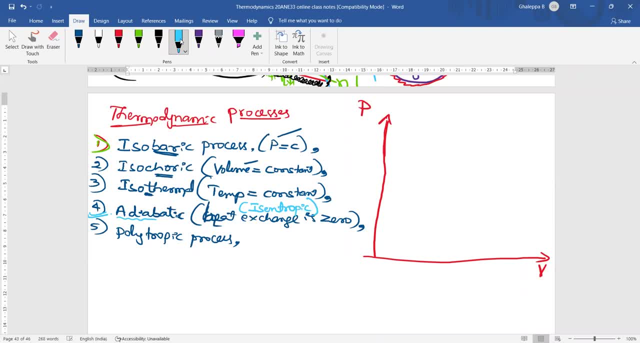 can remember this point: reversible adiabatic is called as isentropic process. so in isentropic process which property remains constant? try to understand, try to split this word isentropy. in this word you are saying one property: pressure, volume, temperature, enthalpy, entropy, like 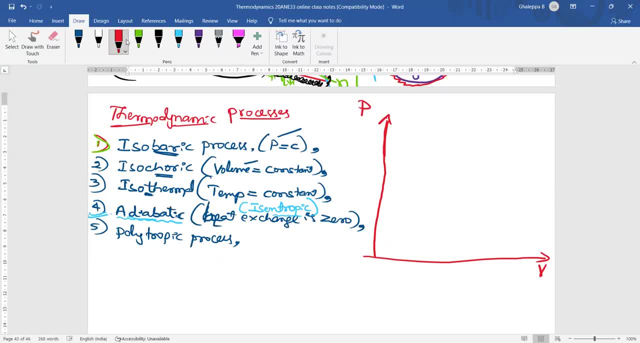 see? here you can see one property. what is the property? entropy? entropy is also a property, just like pressure. pressure is also property, volume is property, temperature is property. so entropy is constant. the process in which entropy is constant throughout the process or during the process, that process is called. 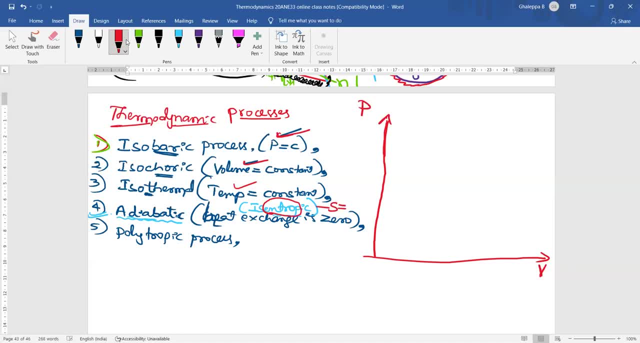 process. okay then, particularly: s is equal to constant. make other thing. okay, I will use this concept in solving numericals. okay. so coming back to the PV diagram, okay, first I will represent isobaric process in the Pew diagram. isobaric means constant pressure, iso means same. it is a Greek. 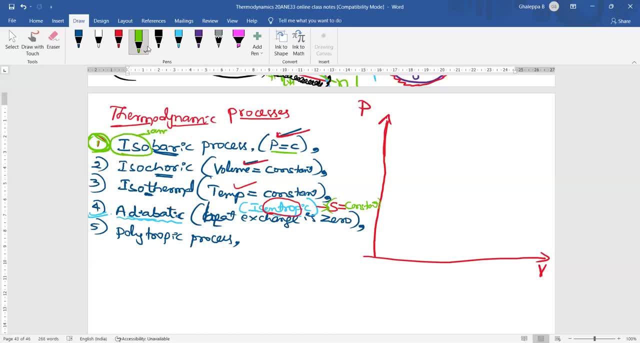 word for downstream Iso means same or constant, so process in which the pressure is constant or pressure is the same, so that process is called isobaric process. so how to represent on the view diagram: P is pressure, V iso Alu. how to represent on the diagram. 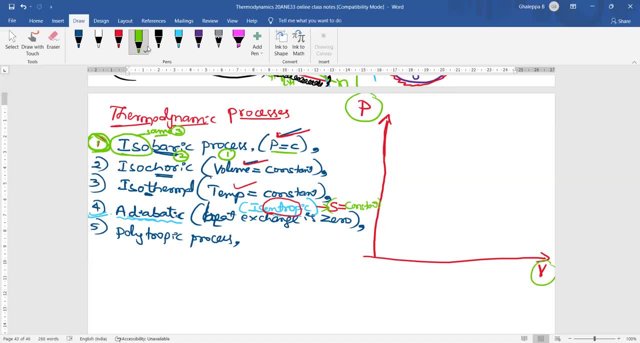 constant pressure. horizontal line or vertical line constant pressure: for example, it is 0, 0 bar, 1 bar, 2 bar, 3 bar, 4 bar, 5 bar, so on. and during the process it should be constant. so how will you represent process here? horizontal line: 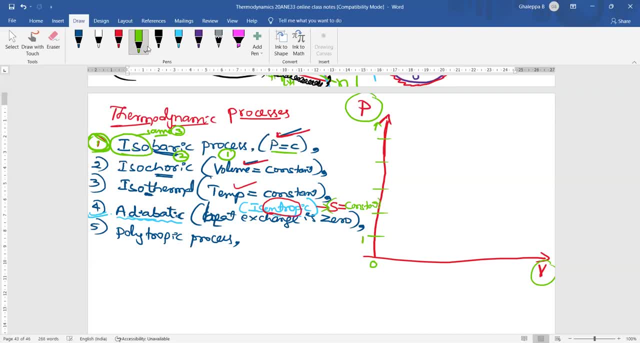 or vertical line. it should be constant. 1 bar, 2, 3. that's an example. I am telling you: okay, it should be constant. the process is at 1 bar, isobaric process it 1 bar. so you should have to represent it with horizontal line. so this is: 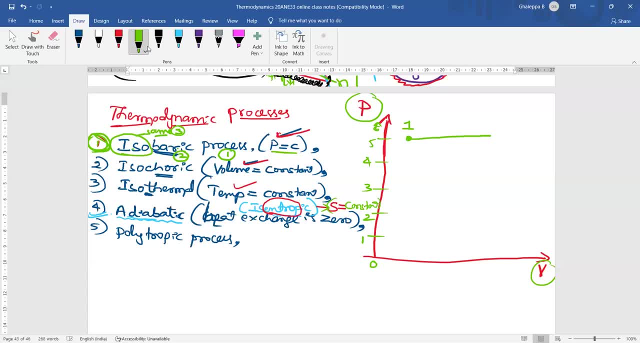 beginning of the point, beginning of the process, point 1. this is end of the process. point 2: so during 1 to 2, the pressure is constant. so in this situation, the pressure is constant. so in this situation, the pressure is constant. so in this, so in this situation, the pressure is constant. so in this graph, how much is a pressure? how much is? 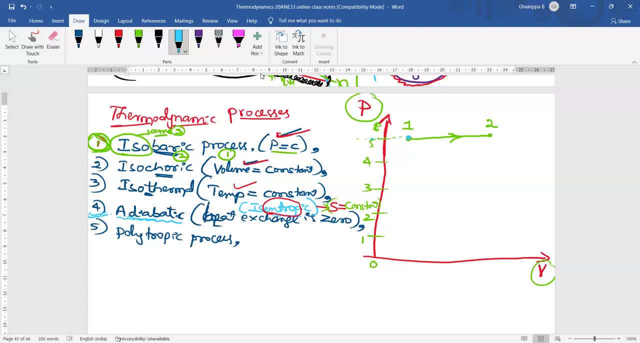 graph. how much is a pressure? how much is graph? how much is a pressure? how much is a pressure at point number one? okay. how a pressure at point number one? okay. how a pressure at point number one? okay. how much is a pressure at the end of the? 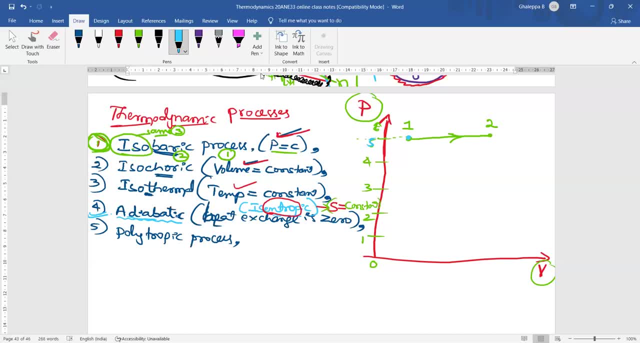 much is a pressure at the end of the much is a pressure at the end of the process, after the end of the first 5 bar process, after the end of the first 5 bar process, after the end of the first 5 bar. so here it is. there is constant. 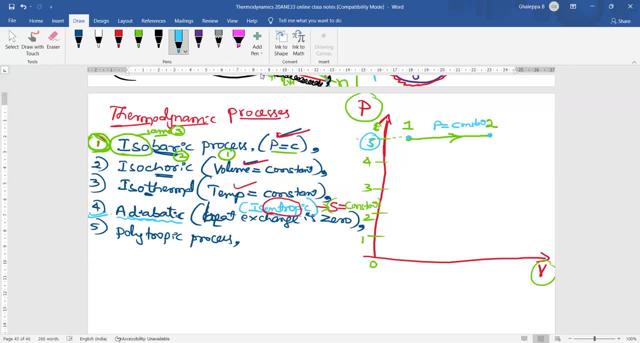 so here it is, there is constant. so here it is, there is constant constant pressure that is 5 bar. okay. so, constant pressure, that is 5 bar. okay. so, constant pressure, that is 5 bar, okay. so, dear students, remember point number. dear students, remember point number 1. 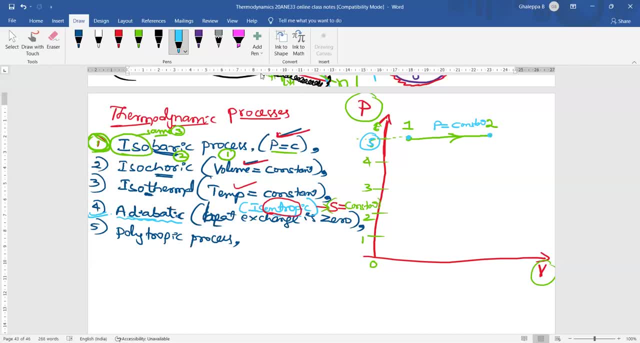 dear students, remember point number 1. dear students, remember point number 1. is initial point of the process or final? is initial point of the process or final? is initial point of the process or final? point point number one: it is initial point. point number one: it is initial. 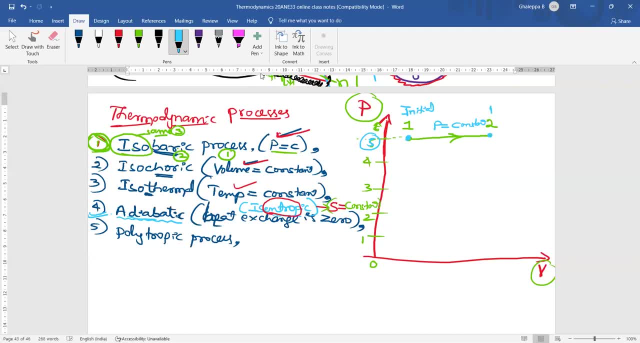 point, point number one. it is initial point. point number two: it is a final point. point number two: it is a final point, point number two: it is a final point okay. and if you take the volume point okay and if you take the volume point, okay, and if you take the volume, v1 is initial volume, v2 volume at point. 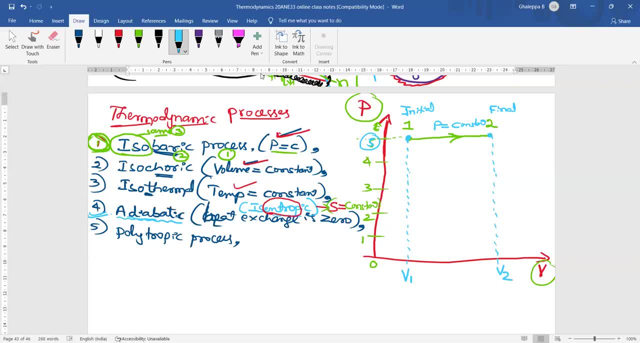 v1 is initial volume. v2 volume at point v1 is initial volume. v2 volume at point number two. now, if you plot a graph number two, now, if you plot a graph number two, now, if you plot a graph of this curve, this line v1 is initial. 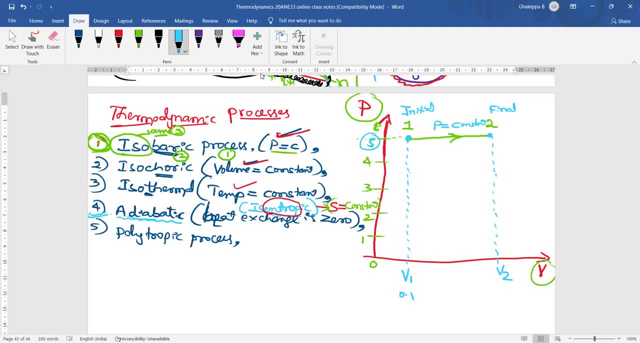 of this curve. this line v1 is initial of this curve. this line v1 is initial volume: it may be 0.1 and v2 may be 0.5. volume: it may be 0.1 and v2 may be 0.5. 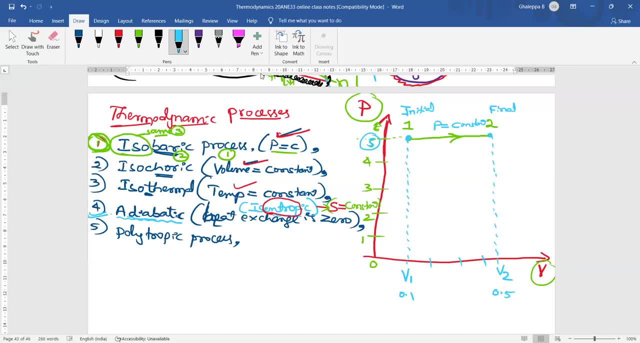 volume it may be 0.1 and v2 may be 0.5. point 1. point 2. point 3. point 4: like this: point 1. point 2. point 3. point 4: like this: point 1. point 2. point 3. point 4: like this: okay, this is xx, 0.1. point 2. point 3. 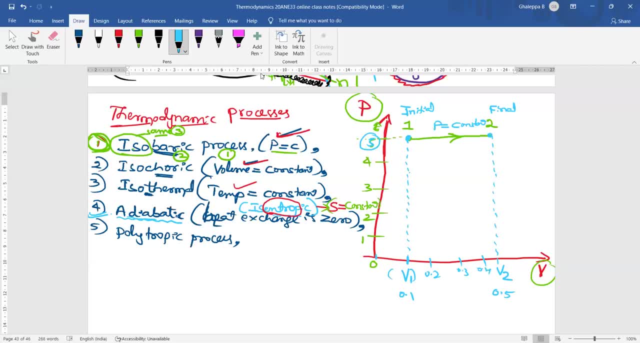 okay, this is xx 0.1, point 2, point 3, point 4. okay, this is xx 0.1, point 2, point 3, point 4, just an example. I am telling you, okay, just an example. I am telling you okay, just an example. I am telling you, okay, these values will be given in the. 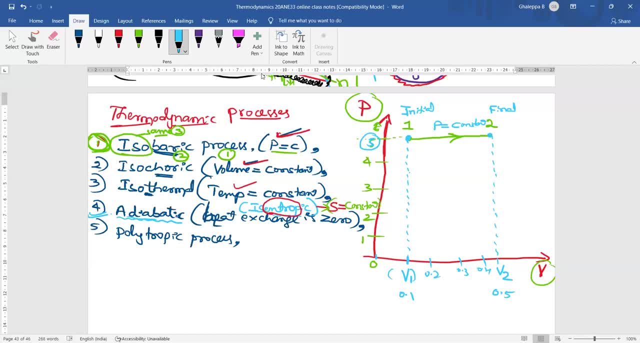 these values will be given in the. these values will be given in the numericals, okay, and this you know first, numericals, okay, and this you know first. numericals, okay, and this you know. first point is: you have to write pressure is. point is: you have to write pressure is. 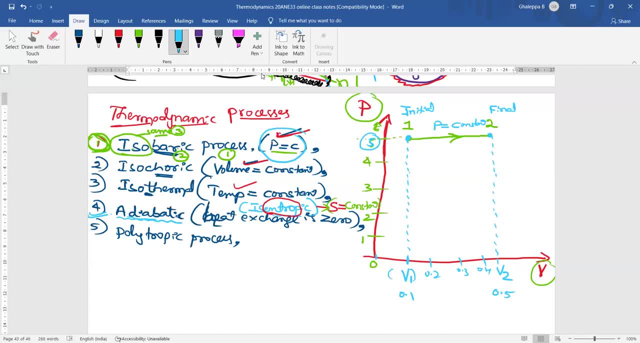 point is you have to write: pressure is equal to constant. second point: is the equal to constant. second point: is the equal to constant. second point is: the process should be represented with. process should be represented with. process should be represented with horizontal line. and here also you write: 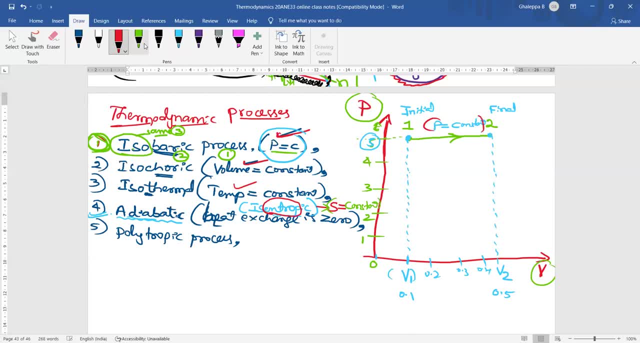 horizontal line, and here also you write horizontal line, and here also you write pressure constant. so during this process, pressure constant. so during this process, pressure constant. so during this process, the pressure is at the initial point, it, the pressure is at the initial point, it, the pressure is at the initial point, it is P 1 and the final point, it is P 2. so 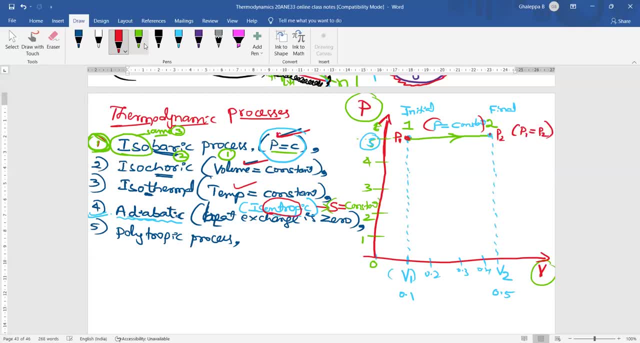 is P 1 and the final point it is P 2. so is P 1 and the final point it is P 2. so P 1 is equal to P 2 during this process. P 1 is equal to P 2 during this process. 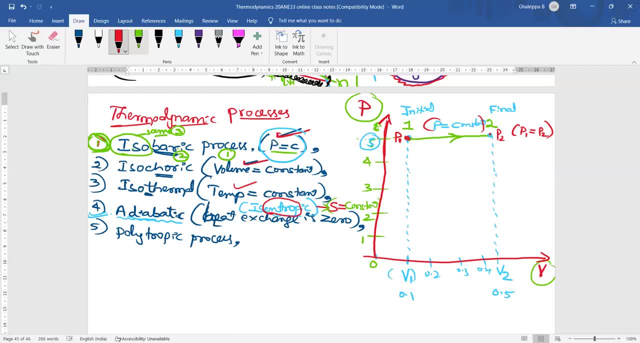 P 1 is equal to P 2 during this process. okay, this is second the one more point. okay, this is second the one more point. okay, this is second the one more point. what you need to remember here is n. what you need to remember here is n. 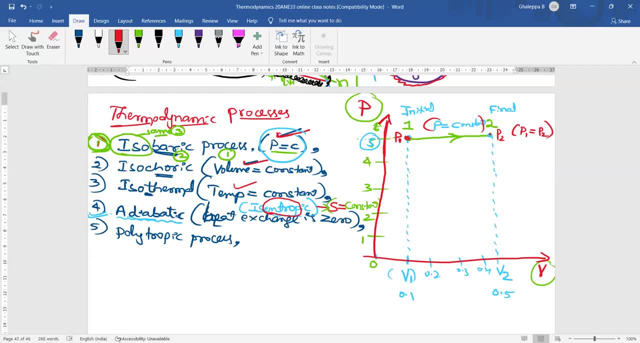 what you need to remember here is n. value n, that is polytropic index. value n, that is polytropic index. value n, that is polytropic index. polytropic index is n adiabatic index. polytropic index is n- adiabatic index. 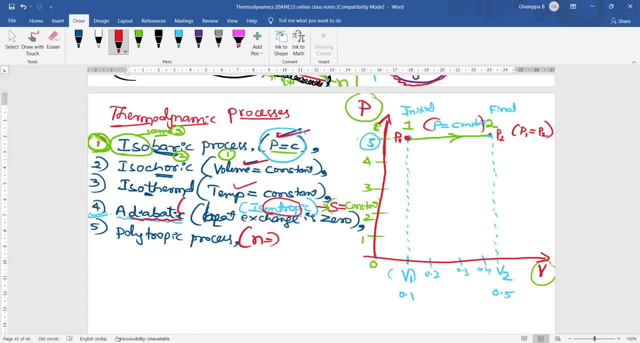 polytropic index is n. adiabatic index will be represented. with which symbol will be represented? with which symbol will be represented? with which symbol? symbol for adiabatic index area- gamma symbol for adiabatic index area- gamma. symbol for adiabatic index area, gamma, gamma. okay, remember adiabatic index. 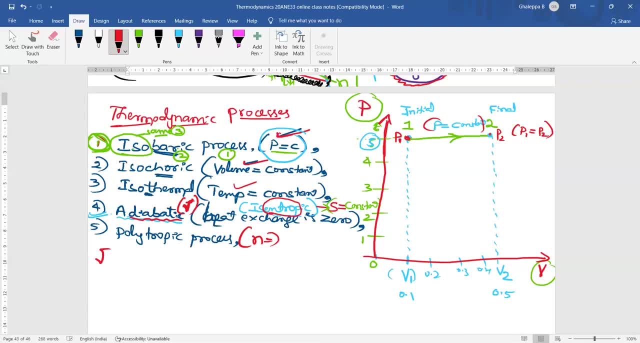 gamma. okay, remember, adiabatic index- gamma. okay, remember, adiabatic index will be represented symbol gamma. like will be represented symbol gamma. like will be represented symbol gamma. like this gamma polytropic process or this gamma polytropic process, or this gamma polytropic process or polytropic index will be represented. 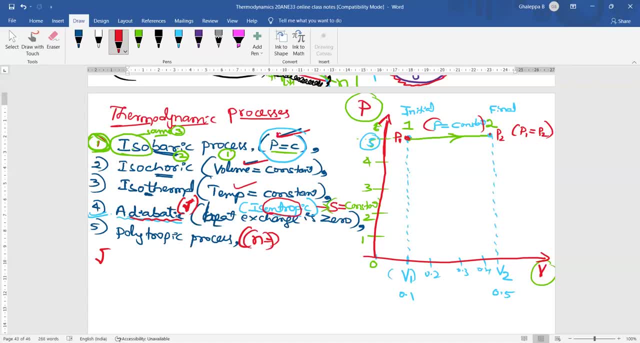 polytropic index will be represented. polytropic index will be represented with letter n- small n okay. lowercase N. with letter n- small n okay. lowercase N. with letter n- small n okay. lowercase N, okay. next, and here the value of n is 0- okay. next, and here the value of n is 0. 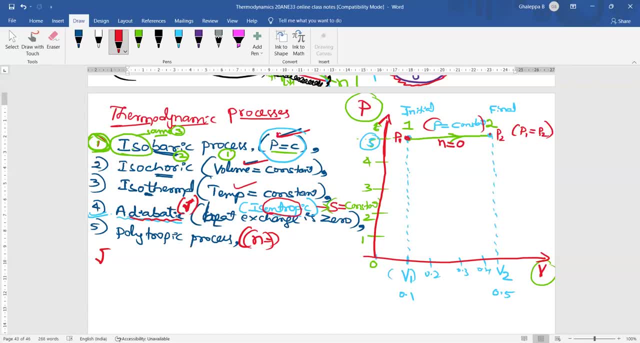 okay. next, and here the value of n is 0. keep in mind if someone asked you in. keep in mind, if someone asked you in. keep in mind. if someone asked you in the interview what is a polytropic index, the polytropic index for isobaric process- you should say n is. 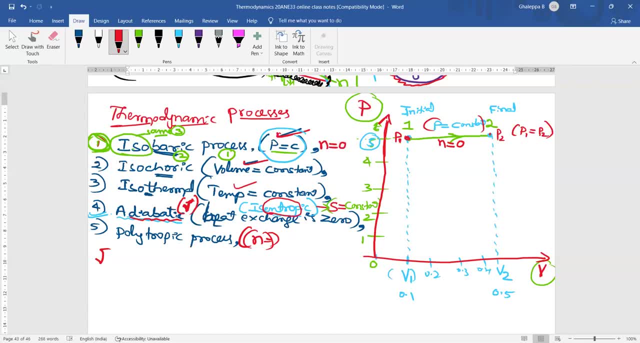 for isobaric process. you should say: n is for isobaric process. you should say: n is equal to 0. n is equal to 0- okay, all equal to 0. n is equal to 0- okay, all equal to 0. n is equal to 0- okay. all these are all new points, new concept. you. 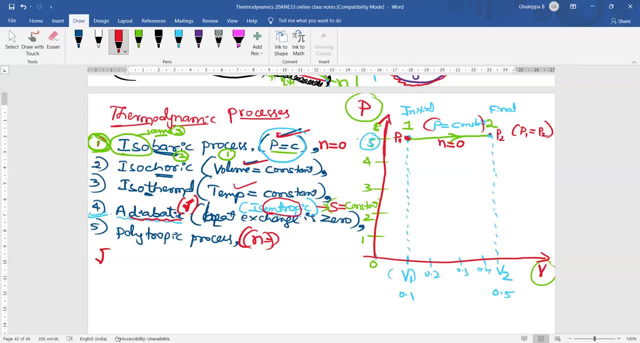 these are all new points, new concept. you- these are all new points, new concept you must remember: okay within thermodynamics, okay within thermodynamics, okay within thermodynamics, okay next. what we need to remember here, okay next. what we need to remember here, okay next. what we need to remember here is: 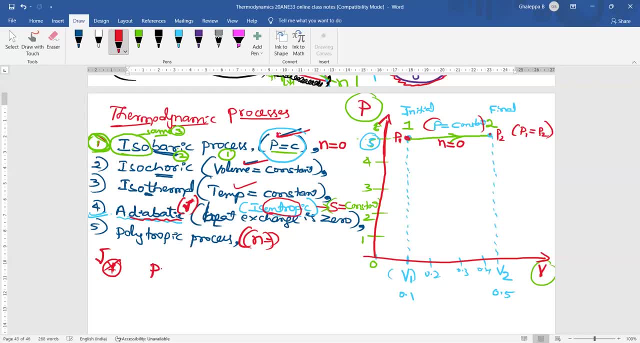 is is okay. I will give one hint okay. PV to the okay. I will give one hint okay. PV to the okay. I will give one hint okay. PV to the power of gamma, or PV to the power of N. power of gamma or PV to the power of N. 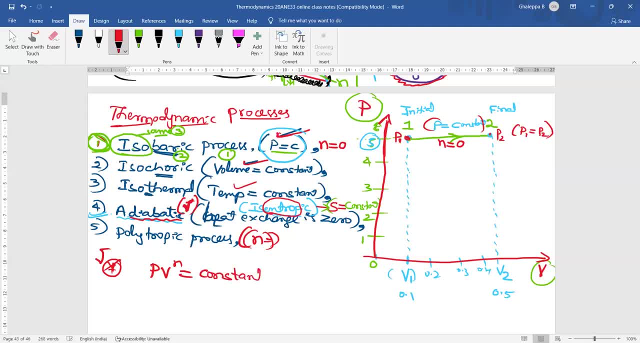 power of gamma or PV to the power of N is equal to constant. you remember, this is equal to constant. you remember, this is equal to constant. you remember this. okay, you can ask a question. so this? okay, you can ask a question. so this: okay, you can ask a question. so this equation, it is for which process? so, equation it is for which process. so equation, it is for which process. so someone has asked you in the last class. someone has asked you in the last class. someone has asked you in the last class: sir, how, what she? why should you write? sir, how, what she? why should you write? 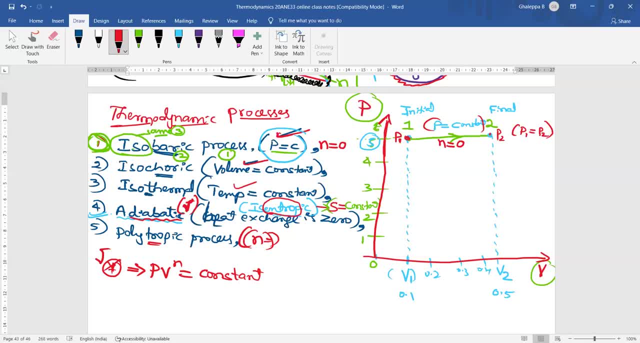 sir, how, what she? why should you write for polytropic? which property remains for polytropic? which property remains for polytropic? which property remains constant? if they ask for definition of constant, if they ask for definition of constant, if they ask for definition of polytropic process, so polytropic process. 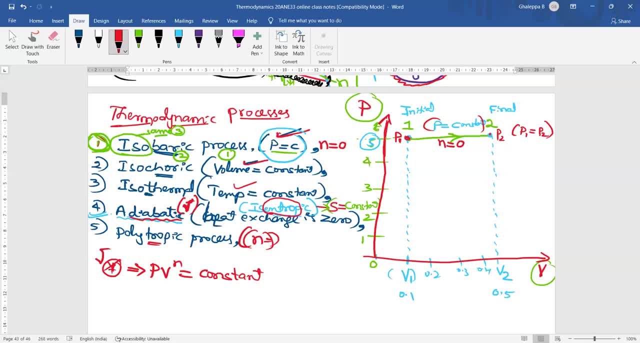 polytropic process, so polytropic process. polytropic process, so polytropic process. it is a process which satisfy, or it is a process which satisfy, or it is a process which satisfy or which obey the law. PV to the power of N is which obey the law. PV to the power of N is: 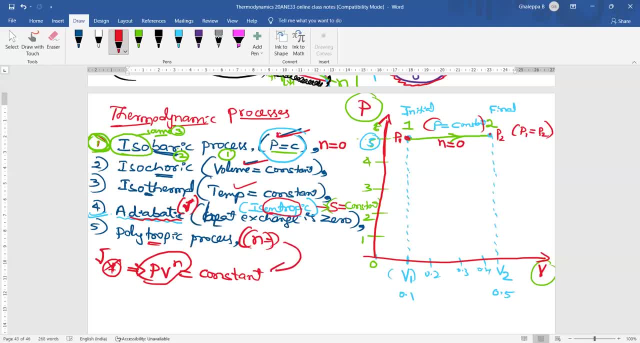 which obey the law. PV to the power of N is equal to constant. okay, what is the equal to constant? okay, what is the equal to constant? okay, what is the definition of polytropic process and definition of polytropic process and definition of polytropic process? and here there is: property is not constant. 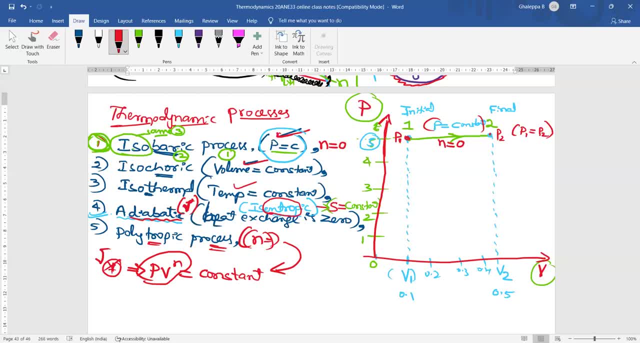 here, there is. property is not constant. here, there is, property is not constant. any property will not be constant here. any property will not be constant here. any property will not be constant here. PV to the power of N. the law is called as. PV to the power of N. the law is called as. 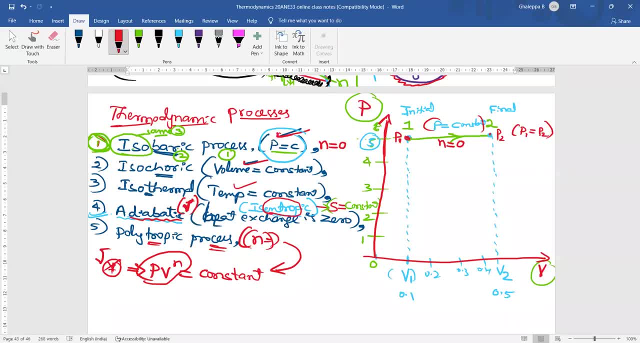 PV to the power of N. the law is called as polytropic process, any process which polytropic process, any process which polytropic process, any process which obey. we satisfy the law PV to the power. obey. we satisfy the law, PV to the power. obey we satisfy the law, PV to the power of N. okay, do your students? I think you. 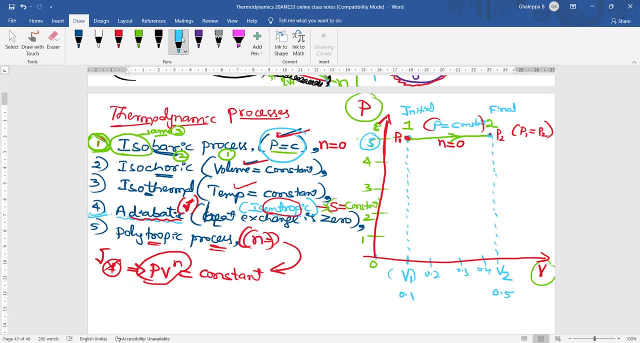 of N. okay, do your students, I think you of N. okay, do your students. I think you know a little bit of mathematics. know a little bit of mathematics. know a little bit of mathematics. knowledge here: if you substitute n, is knowledge here. if you substitute n, is knowledge here. if you substitute n is equal to 0, what we'll get in this? 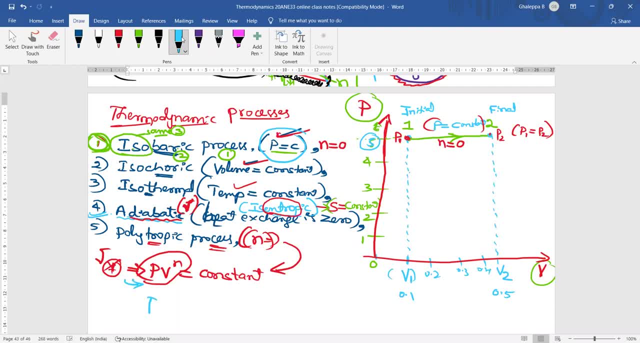 equal to 0. what we'll get in this: equal to 0. what we'll get in this equation: P V to the power of 0 is equal. equation P V to the power of 0 is equal. equation P V to the power of 0 is equal to constant. what we'll get: V to the. 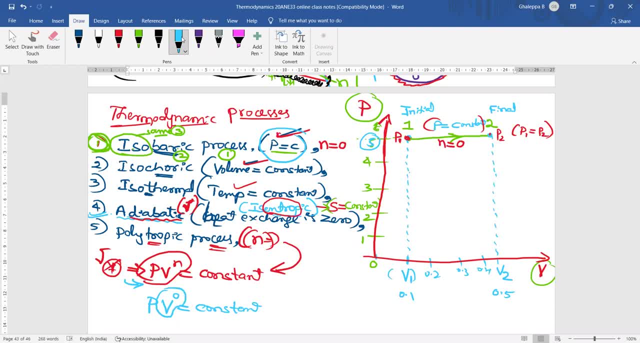 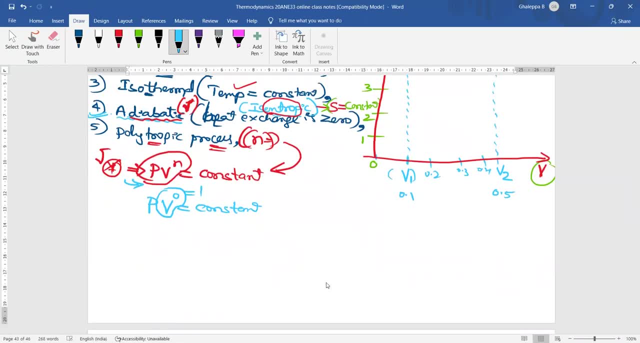 to constant. what we'll get V to the to constant. what we'll get V to the power of 0 is what? anything? any value to power of 0 is what? anything? any value to power of 0 is what anything. any value to the power of 0 is equal to 1: 1 pressure. 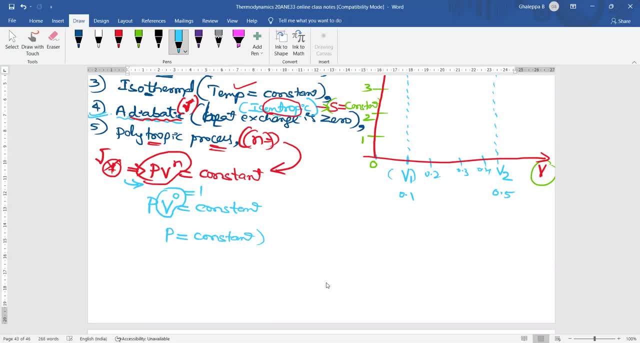 the power of 0 is equal to 1. 1 pressure: the power of 0 is equal to 1. 1 pressure is equal to constant unit. that is, the is equal to constant unit. that is, the is equal to constant unit. that is the reason I said here: n is equal to 0. why? 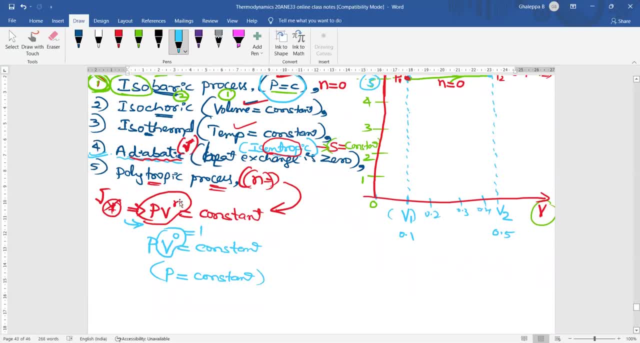 reason I said here n is equal to 0. why reason I said here n is equal to 0? why he said n is equal to 0. if you put n, is he said n is equal to 0. if you put n, is he said n is equal to 0. if you put n is equal to 0, in this equation you will get: 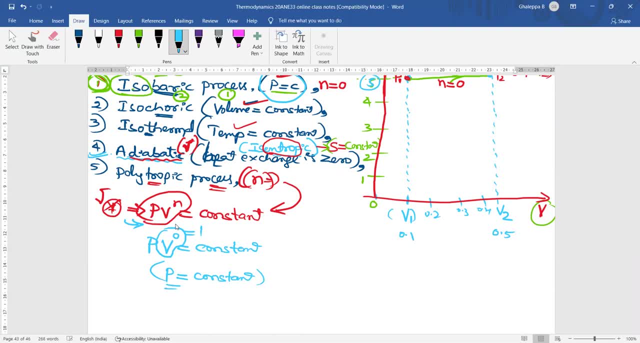 equal to 0 in this equation, you will get equal to 0. in this equation, you will get: the pressure is equal to constant. okay, the pressure is equal to constant. okay, the pressure is equal to constant. okay. now second process: isochoric, isochoric. now second process: isochoric, isochoric. 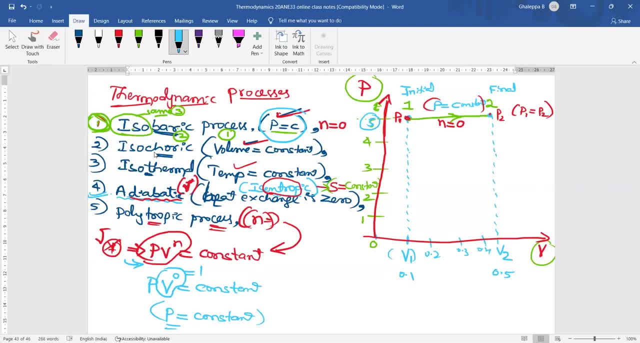 now second process: isochoric, isochoric process. so isochoric process is volume process. so isochoric process is volume process. so isochoric process is volume is equal to constant, so volume is on is equal to constant. so volume is on is equal to constant, so volume is on x-axis. so during the process, the volume, 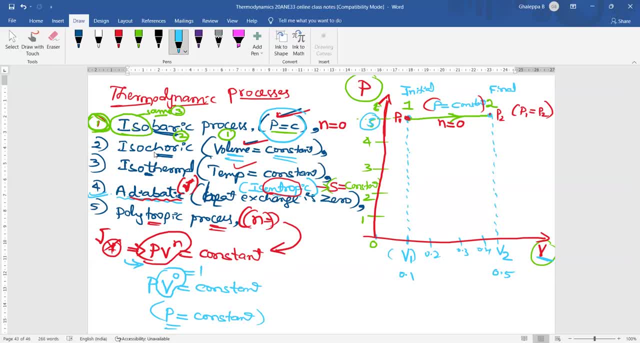 x-axis, so during the process the volume x-axis, so during the process. the volume is 0.1 meter cube. so then means initial is 0.1 meter cube. so then means initial is 0.1 meter cube. so then means initial volume is 0.1 meter cube. final volume is: 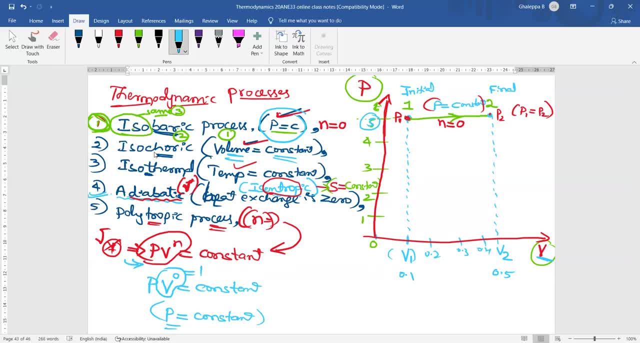 volume is 0.1 meter cube. final volume is. volume is 0.1 meter cube, final volume is also 0.1 meter cube. and how will you also 0.1 meter cube and how will you also 0.1 meter cube and how will you represent in the pew diagram vertical? 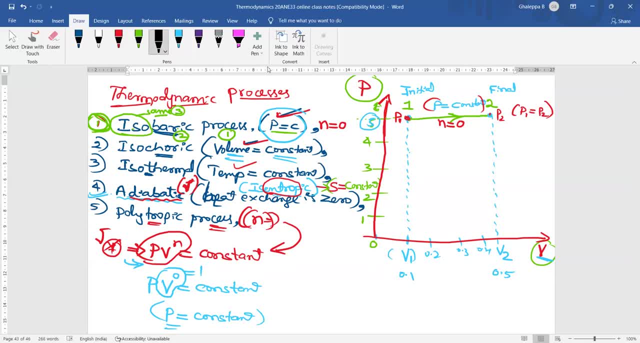 represent in the pew diagram: vertical. represent in the pew diagram: vertical line or horizontal line. initial point line or horizontal line. initial point line or horizontal line. initial point and final point should lies on the same and final point should lies on the same and final point should lies on the same line. vertical or horizontal? horizontal. 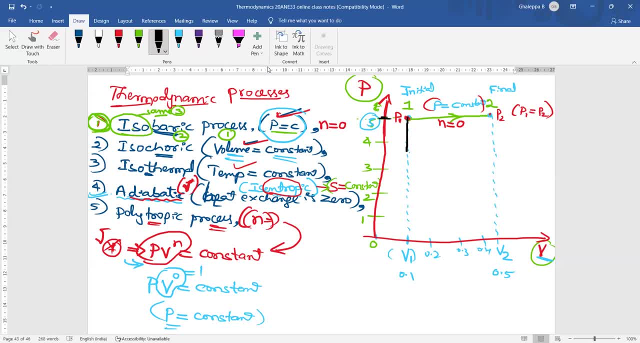 line, vertical or horizontal. horizontal line vertical or horizontal horizontal. it is for isobaric horizontal. is it is for isobaric horizontal. is it is for isobaric horizontal is presumably constant. I need volume presumably constant. I need volume presumably constant. I need volume constant. what we can write, so what? 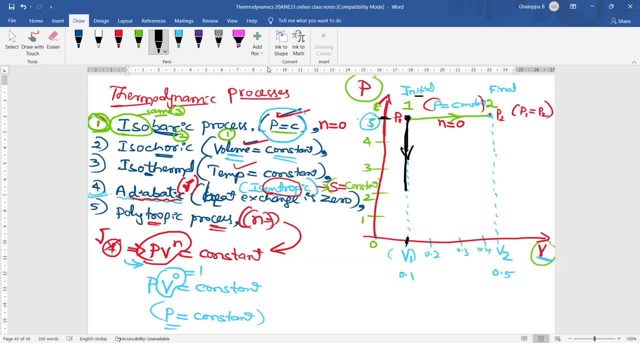 constant what we can write, so what constant what we can write, so what. what constant what we can write, so what, what. so point number one is initial point, so point number one is initial point. so point number one is initial point. point number two is final point. so now 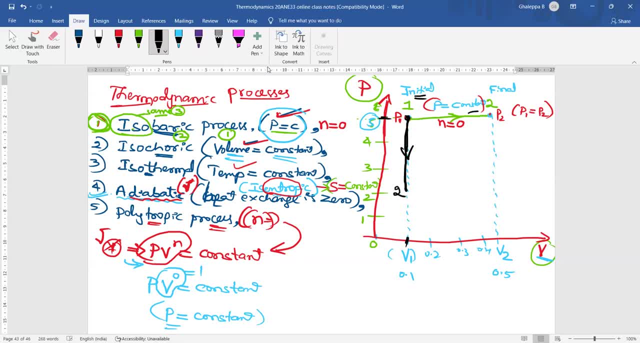 point number two is final point. so now, point number two is final point. so now, you do not look, do not look at this one. you do not look, do not look at this one. you do not look, do not look at this one to two. it is over this for isobaric. 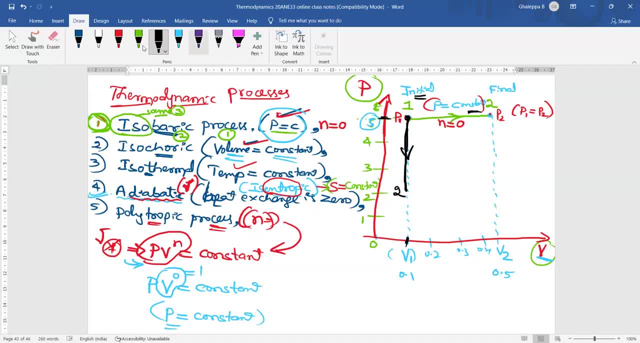 to two. it is over this for isobaric to two. it is over this for isobaric only. you look at only for this vertical, only you look at only for this vertical, only you look at only for this vertical line. so in this vertical line, initial. 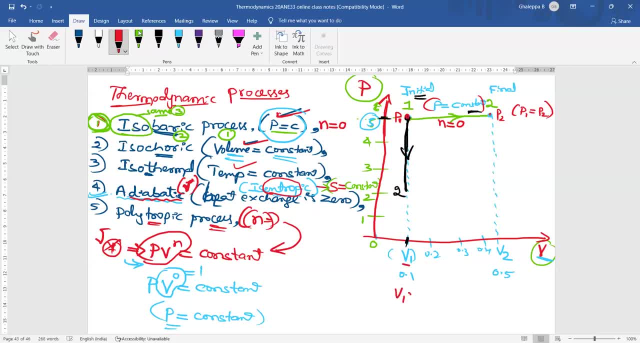 line. so in this vertical line, initial line. so in this vertical line, initial point is v1: okay, v1 is equal to 0.1. so point is: v1: okay, v1 is equal to 0.1. so point is v1, okay, v1, okay, v1. so here volume is same. the process ends at. 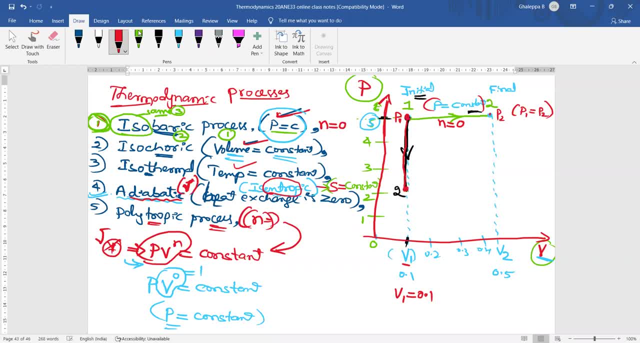 here, volume is same. the process ends at here. volume is same. the process ends at point number two. what is a volume at point number two? what is a volume at point number two? what is a volume at point number two? 0.1. that is 0.1, okay. 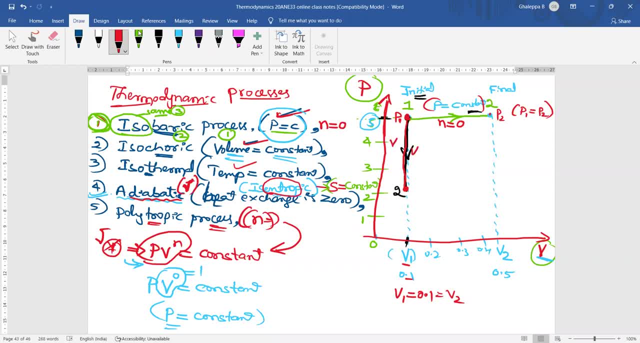 point number two: 0.1, that is 0.1. okay, point number two: 0.1, that is 0.1. okay, here, volume is equal to constant. you, here, volume is equal to constant. you, here, volume is equal to constant. you need to write, we need to write the. 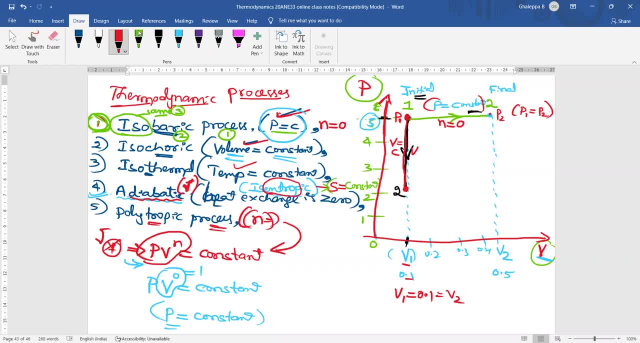 need to write, we need to write, the need to write, we need to write. the volume is equal to constant and the volume is equal to constant, and the volume is equal to constant. and the next point is n value. what is a n value? next point is n value: what is a n value? 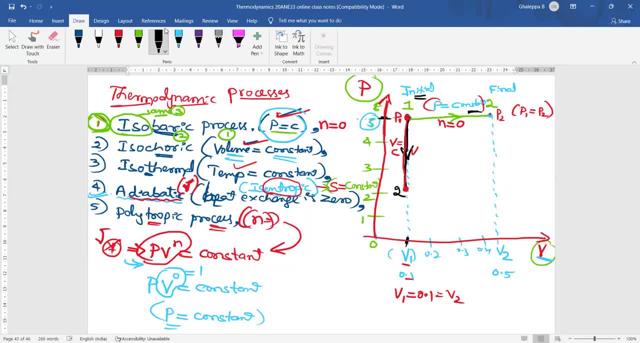 next point is n value. what is a n value for this isochoric process? is n is equal for this isochoric process is n is equal for this isochoric process is n is equal to infinity. you start from 0- here is a to infinity. you start from 0, here is a. 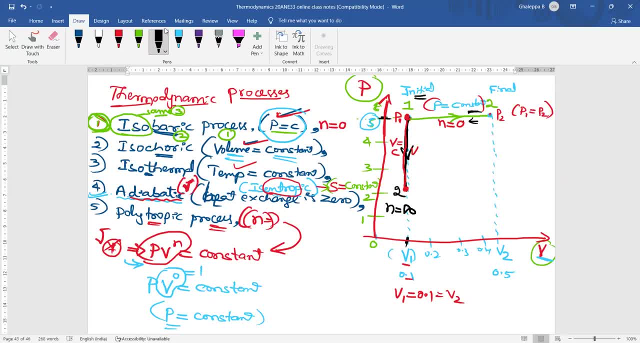 to infinity. you start from 0. here is a zero value: 0, 1, 2, 3, 4, 5, 6, so on, and the zero value 0, 1, 2, 3, 4, 5, 6, so on, and the zero value 0, 1, 2, 3, 4, 5, 6, so on, and the last number is infinity. so n is infinity. 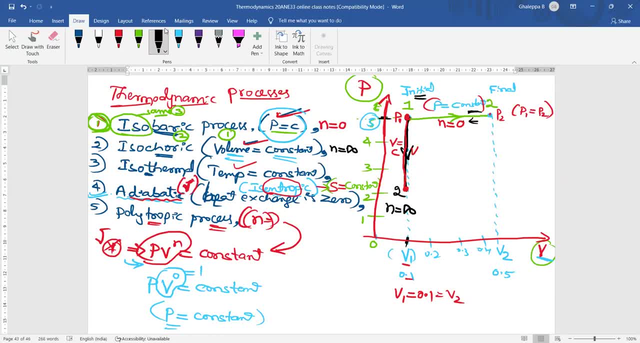 last number is infinity, so n is infinity. last number is infinity, so n is infinity. for isochoric process, remember my dear for isochoric process. remember my dear for isochoric process. remember my dear friends. they may ask you in the friends, they may ask you in the 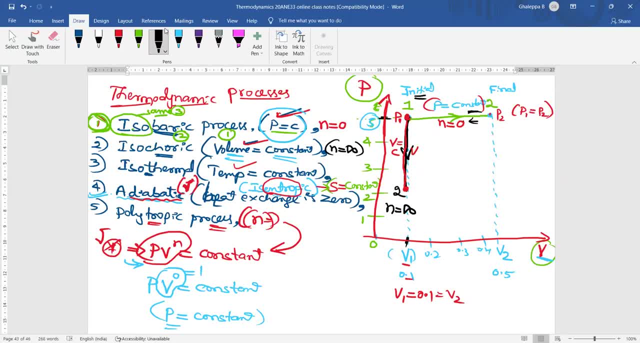 friends. they may ask you in the interviews and all: what is a polytrophic interviews and all? what is a polytrophic interviews and all? what is a polytrophic index for constant volume process? what index for constant volume process? what index for constant volume process? what is a polytrophic index for isochoric? 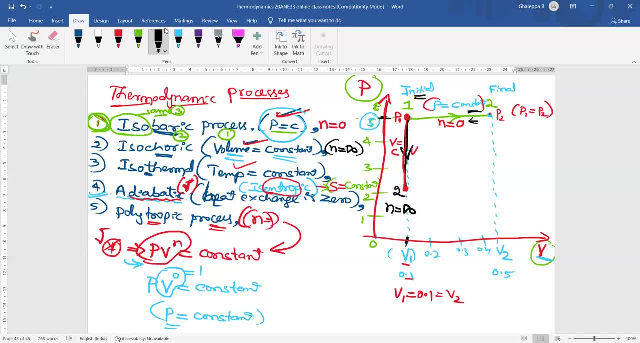 is a polytrophic index for isochoric is a polytrophic index for isochoric process. isochoric is constant volume, so process isochoric is constant volume. so process isochoric is constant volume, so n is equal to infinity. ok, next, ok, next. 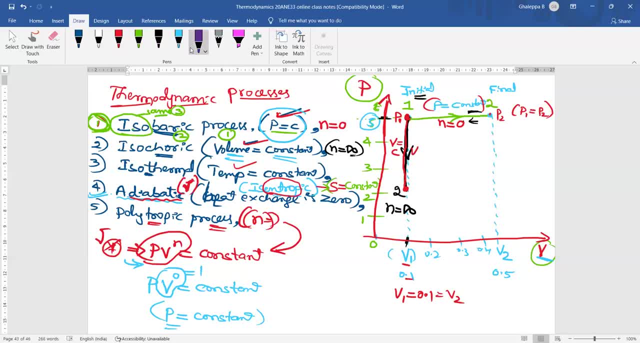 n is equal to infinity, ok, next, ok. next. n is equal to infinity, ok, next, ok, next. third process: isothermal isothermal. third process: isothermal isothermal. third process: isothermal isothermal process. so in this isothermal temperature is constant. so how to write? temperature is constant, so how to write? 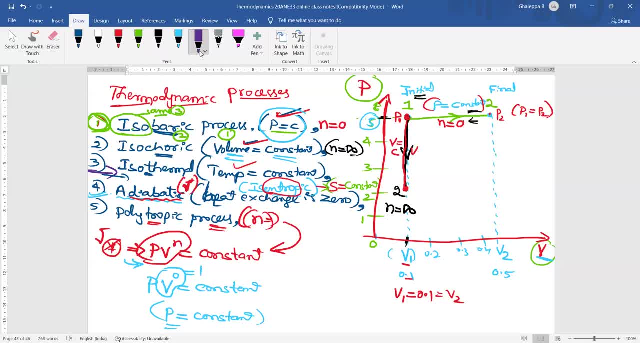 temperature is constant. so how to write how to draw that constant temperature, how to draw that constant temperature, how to draw that constant temperature process in PV diagram. is the assurance process in PV diagram. is the assurance process in PV diagram: is the assurance? one more hint I will do, please listen. 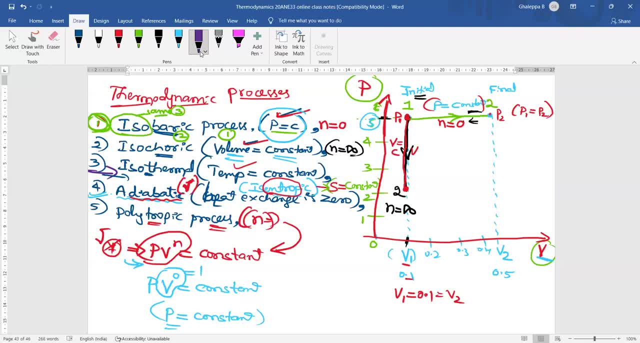 one more hint. I will do, please listen. one more hint, I will do, please listen carefully. this hint is very important. carefully, this hint is very important, carefully. this hint is very important when you are plotting PV diagram. when you are plotting PV diagram, when you are plotting PV diagram. what I'm saying when you are plotting PV. 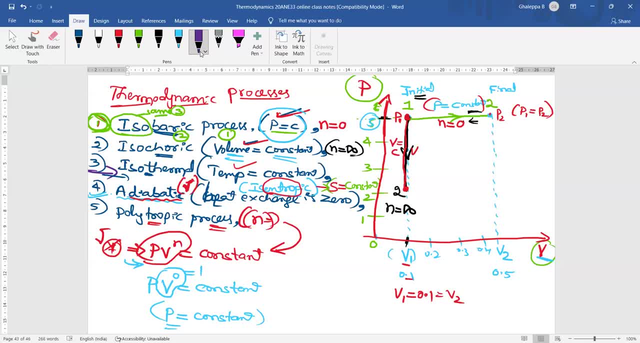 what I'm saying when you are plotting PV, what I'm saying when you are plotting PV diagram for any thermodynamic process diagram, for any thermodynamic process diagram, for any thermodynamic process. you have the other early constant pressure. you have the other early constant pressure. you have the other early constant pressure is a horizontal if it is constant. 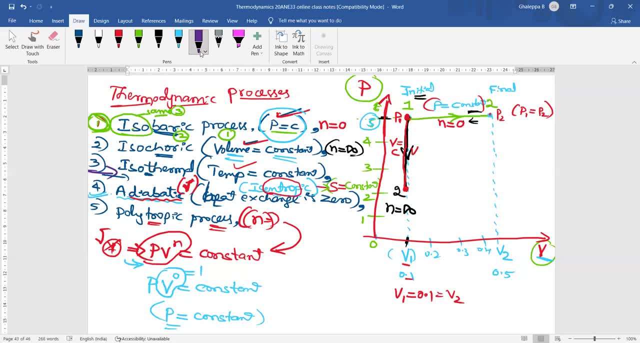 is a horizontal. if it is constant, is a horizontal. if it is constant pressure, you write horizontal. if it is pressure, you write horizontal. if it is pressure, you write horizontal. if it is constant volume, you write vertical. other constant volume, you write vertical. other constant volume, you write vertical. other than these two, other than these two. 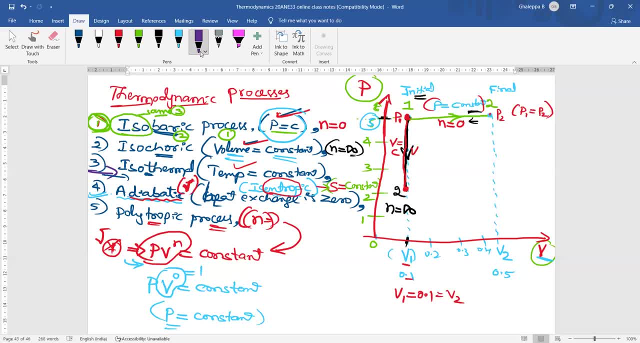 than these two, other than these two, than these two, other than these two, under a constant pressure and constant under a constant pressure and constant under a constant pressure and constant volume bit. if any process is there, draw volume bit. if any process is there, draw volume bit. if any process is there, draw with curve line. that's it. 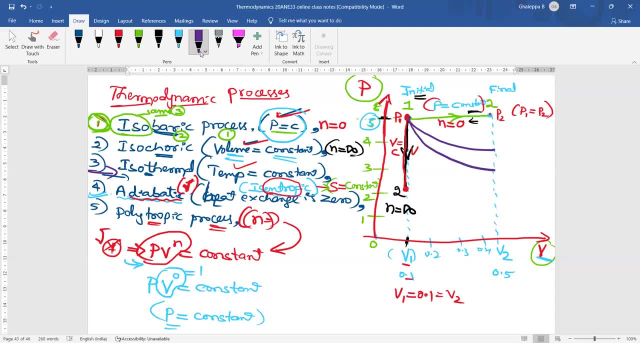 with curve line. that's it with curve line. that's it like this, like this, like this: okay, you draw a curved line like this. so okay, you draw a curved line like this. so okay, you draw a curved line like this. so this is initial. point is 0.1 initial. 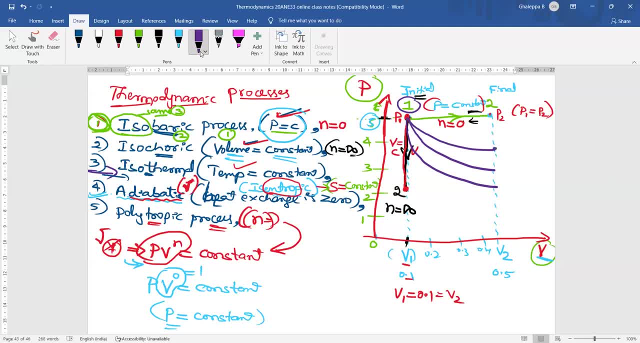 this is initial point. is 0.1 initial. this is initial point. is 0.1 initial point. initial starting or initial process point. initial starting or initial process point. initial starting or initial process. final process is 0.2. final process is 0.2. 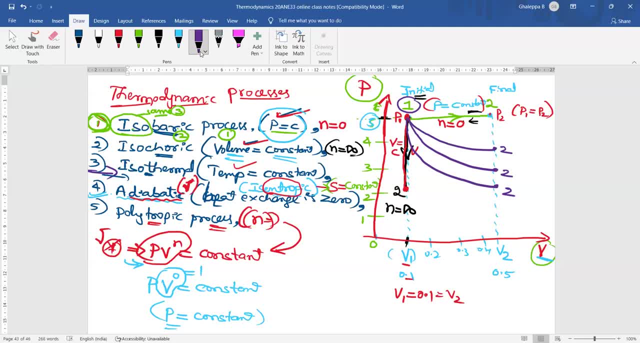 final process is 0.2. our talk to them condition or in a hint. our talk to them condition or in a hint. our talk to them condition or in a hint. and Renner PV diagram of the today, the. and Renner PV diagram of the today, the. 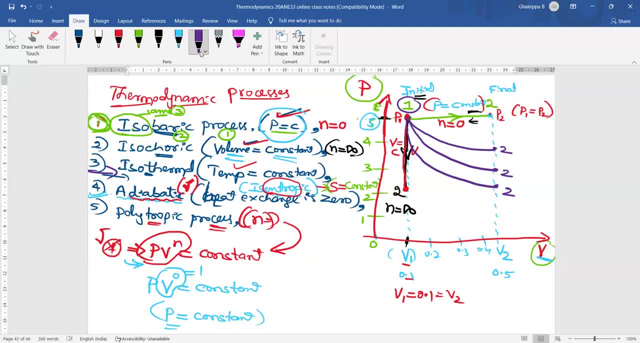 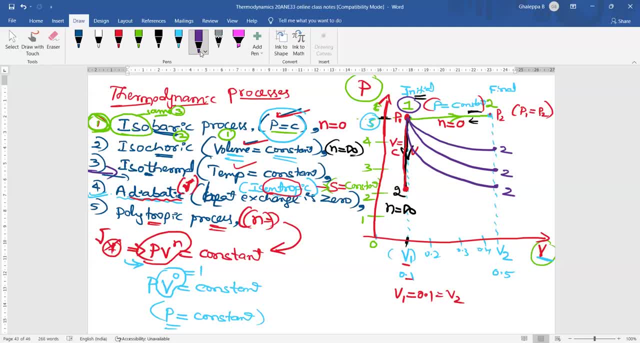 and the word of Andre horizontal, I have, and the word of Andre horizontal I have constant volume and I'd rate vertical constant volume and I'd rate vertical constant volume and I'd rate vertical, and I put you wear it a bit too very and I put you wear it a bit too very. 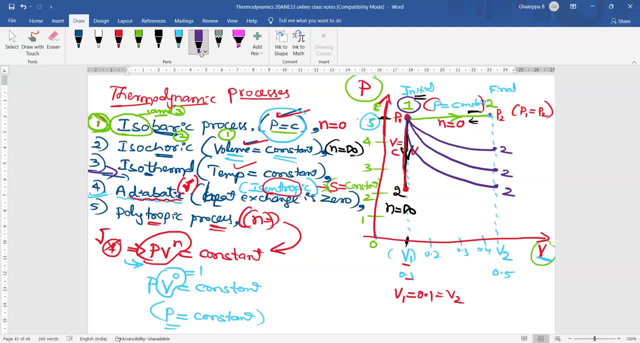 and I put- you wear it a bit too very out of the root thermodynamic process, out of the root thermodynamic process, out of the root thermodynamic process could lower under a temperature, could lower under a temperature, could lower under a temperature. while tropic, adiabatic, isentropic, 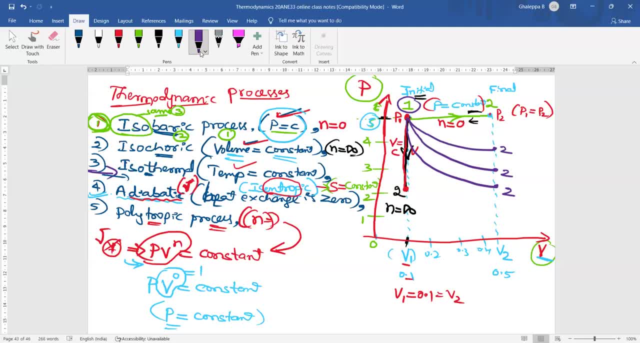 while tropic adiabatic isentropic, while tropic adiabatic isentropic, which are, whichever may be the process, which are, whichever may be the process, which are, whichever may be the process, you have to represent with curved line, you have to represent with curved line. 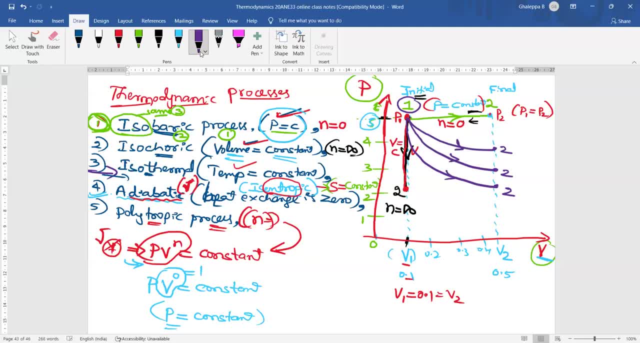 you have to represent with curved line. curved line: okay, this is graph now. curved line. okay, this is graph now curved line. okay, this is graph now. this point is for isothermal. this point is for isothermal. this point is for isothermal- isothermal. now you can ask for what you. 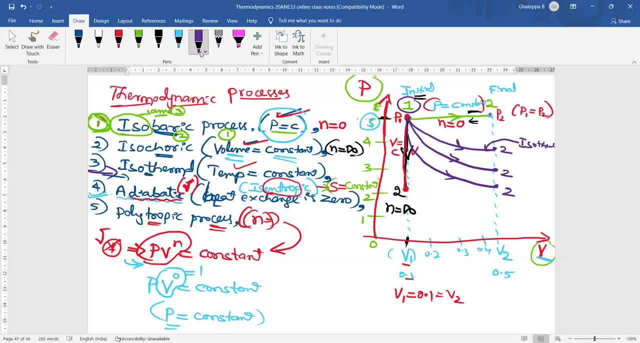 isothermal. now you can ask for what you isothermal. now you can ask for what you should be. the value of n? n is equal to should be. the value of n? n is equal to should be. the value of n? n is equal to 0 for constant pressure. that is isobaric. 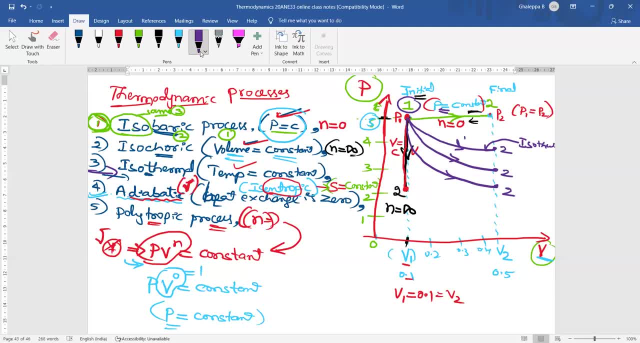 0 for constant pressure that is isobaric. 0 for constant pressure that is isobaric. you should get: n is equal to. you should get. n is equal to. you should get: n is equal to 1 here. 1 here. 1 here n is equal to 1 for isothermal. 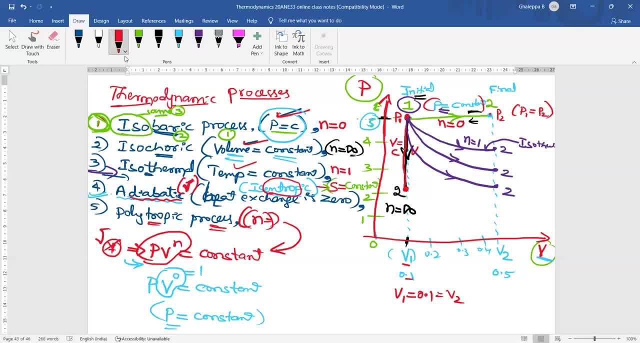 n is equal to 1 for isothermal, n is equal to 1 for isothermal. remember, if you allow value name, particularly remember if you allow value name, particularly remember if you allow value name, particularly: iso thermal n is equal to 1, iso thermal n is equal to 1. 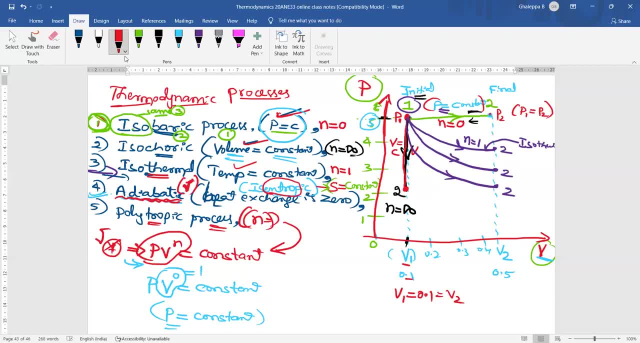 iso thermal n is equal to 1 and next one is adiabatic. fourth one, and next one is adiabatic. fourth one and next one is adiabatic. fourth one. adiabatic, this is first process. adiabatic, this is first process. 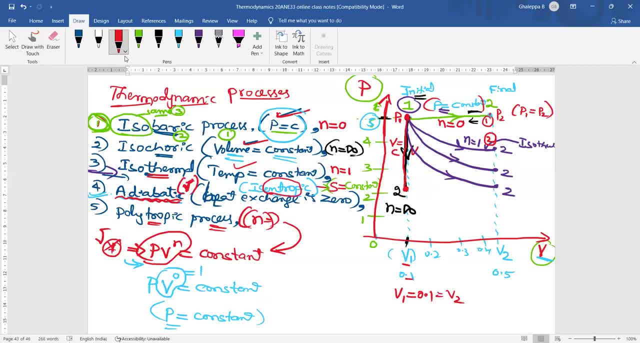 adiabatic. this is first process, second, second, second. third is isothermal, is over. third is isothermal, is over. third is isothermal, is over. fourth one adiabatic pandaga. fourth one adiabatic pandaga. fourth one adiabatic pandaga n value is equal to gamma on the 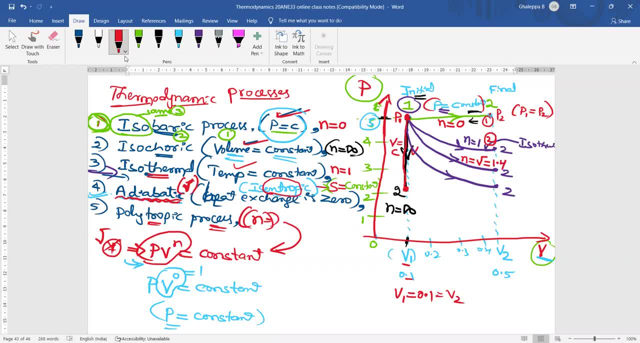 n value is equal to gamma. on the: n value is equal to gamma. on the creativity, that is 1.4. creativity, that is 1.4. creativity, that is 1.4, 1.4. this is for adiabatic, adiabatic, adiabatic. 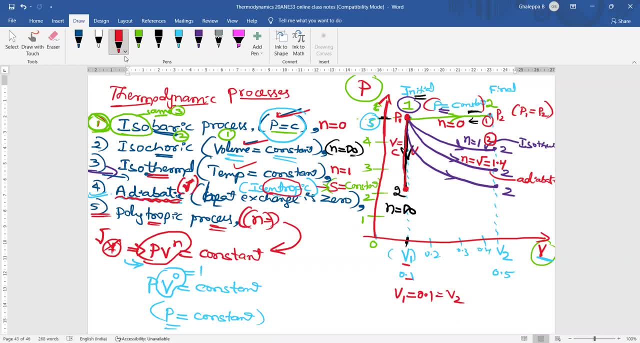 adiabatic adiabatic, adiabatic adiabatic, and last one polytropic, and last one polytropic and last one polytropic. that is for third, that is for third. that is for third. n is equal to n. it is greater than 2. 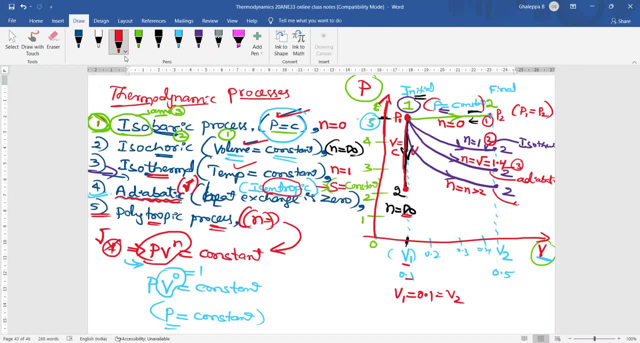 n is equal to n, it is greater than 2. n is equal to n, it is greater than 2, but less than infinity. just like okay. but less than infinity, just like okay. but less than infinity, just like okay, it will be greater than 2. it will be greater than 2. 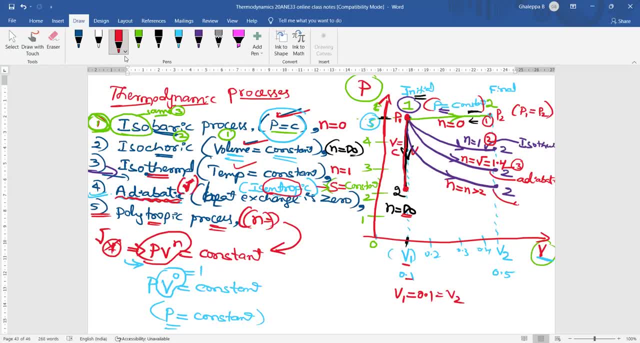 it will be greater than 2. it may be 3, 4, 5, 6, like that. it may be 3, 4, 5, 6, like that. it may be 3, 4, 5, 6, like that. okay, if you don't know the value of n it. 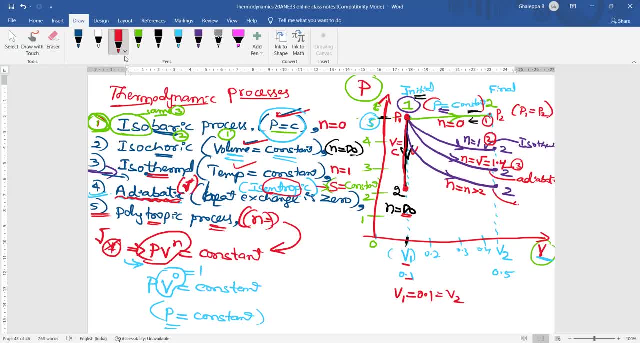 okay. if you don't know the value of n, it okay. if you don't know the value of n, it may be infinity then it is. may be infinity then it is. may be infinity then it is constant volume process. understand, understand, understand. what is the confusion here? 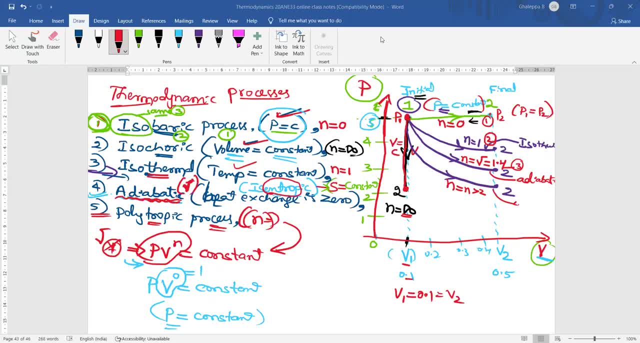 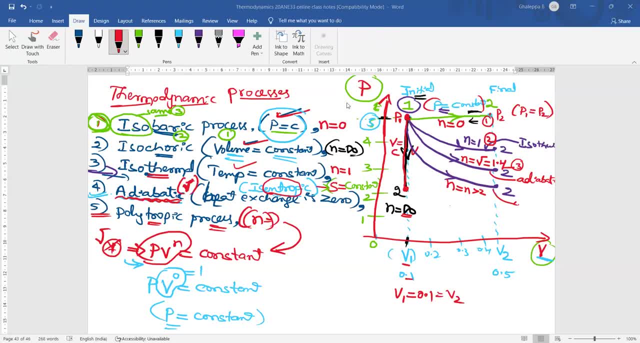 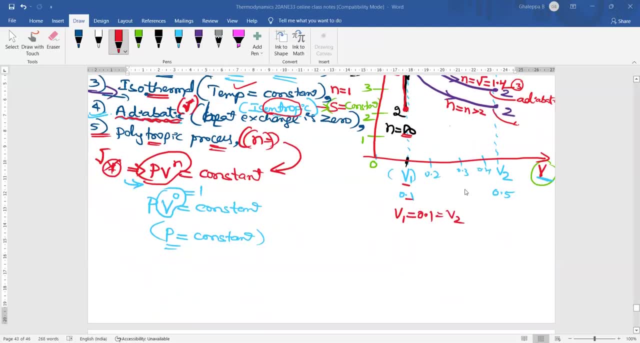 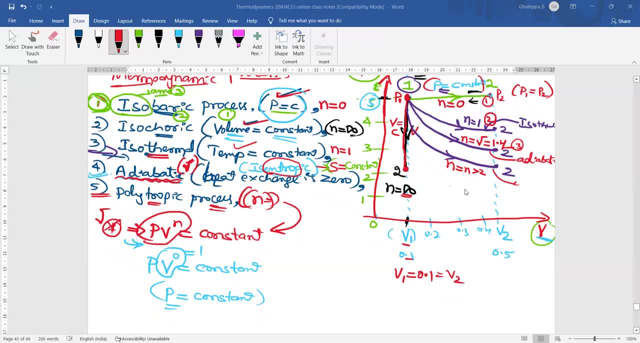 one more time you watch this video and one more time you watch this video and you will get- you will clear all the you will get. you will clear all the you will get. you will clear all the doubts. okay, because this is the first doubts. okay, because this is the first. 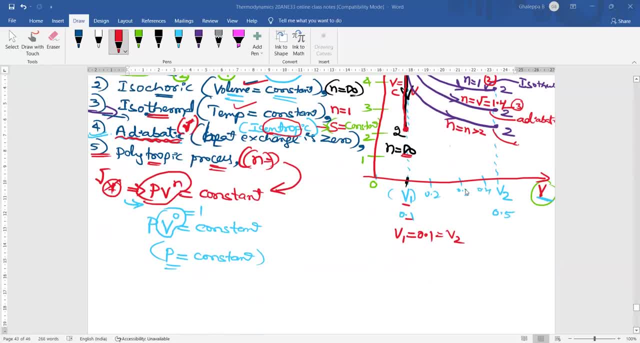 doubts. okay, because this is the first time you are at thermodynamics. you feel time you are at thermodynamics. you feel time you are at thermodynamics, you feel it is little bit tough, you feel it is it is little bit tough, you feel it is it is little bit tough. you feel it is little bit tough. okay, but a terrain. 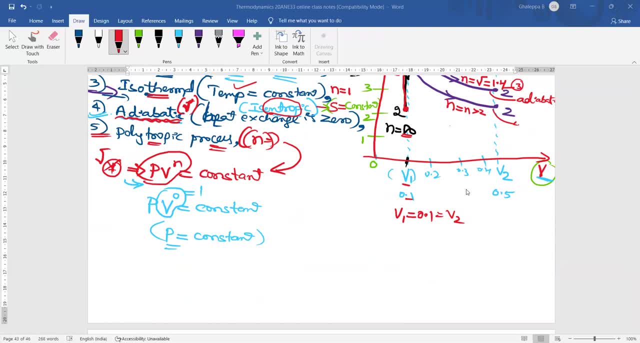 little bit tough, okay, but a terrain. little bit tough okay, but a terrain. okay, now I will write some equations. okay, now I will write some equations. okay, now I will write some equations, equations and dear students first, and the equations and dear students first. and the equations and dear students first. and the best equation, you remember this PV to. 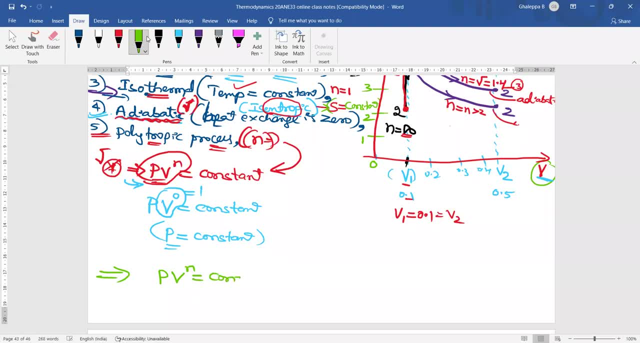 best equation. you remember this PV to best equation. you remember this PV to. the power of n is equal to constant. the power of n is equal to constant. the power of n is equal to constant. first you remember this equation always. first you remember this equation always. first you remember this equation always. you remember this equation all remaining. 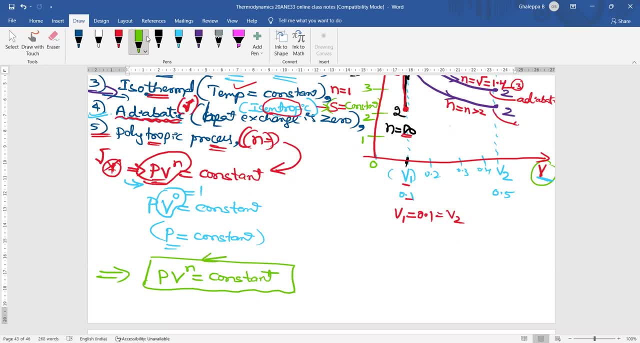 you remember this equation all remaining. you remember this equation. all remaining equations are based on this. I will you. equations are based on this. I will you equations are based on this. I will you hint how to remember if n is equal to 0, if. hint how to remember if n is equal to 0, if. 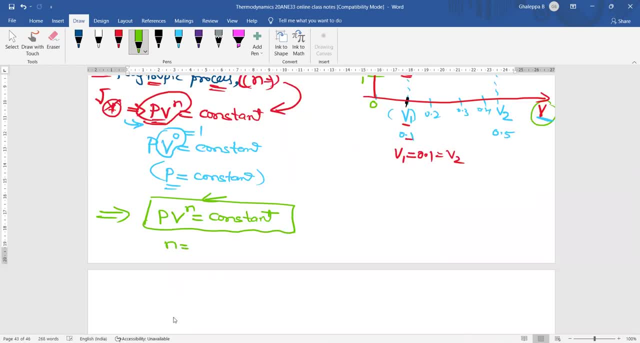 hint: how to remember if n is equal to 0. if you put n is equal to 0, what you will you put n is equal to 0. what you will you put n is equal to 0, what you will get. P is equal to constant. P is equal to. 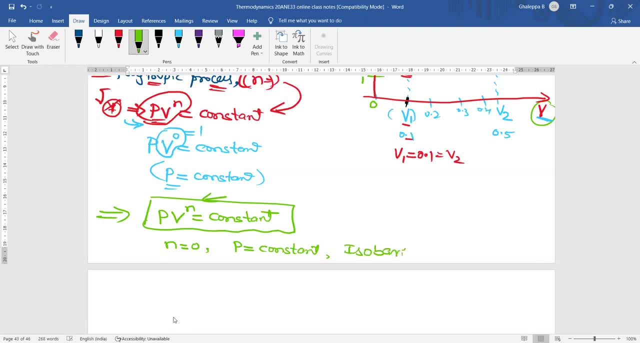 get. P is equal to constant. P is equal to get. P is equal to constant. P is equal to constant means isobaric process. okay, constant means isobaric process. okay, constant means isobaric process. okay, next time again, I will write the same. next time again, I will write the same. 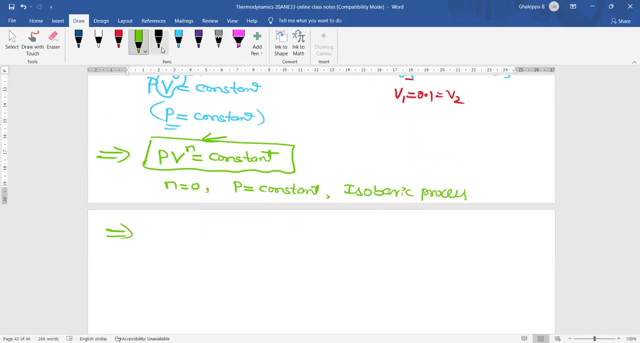 next time again, I will write the same equation. I will write PV to the power of equation. I will write PV to the power of equation. I will write PV to the power of. n is equal to constant. n is equal to constant. n is equal to constant. put n is equal to 1. okay, if you put n is. 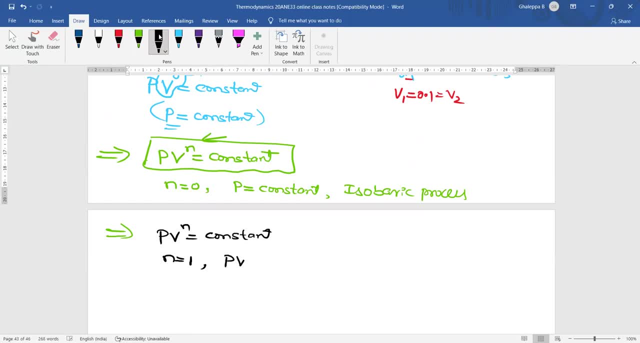 put n is equal to 1. okay, if you put n is put n is equal to 1. okay, if you put n is equal to 1, what you will get, you will equal to 1. what you will get, you will equal to 1. what you will get, you will get. equation: PV is equal to constant. 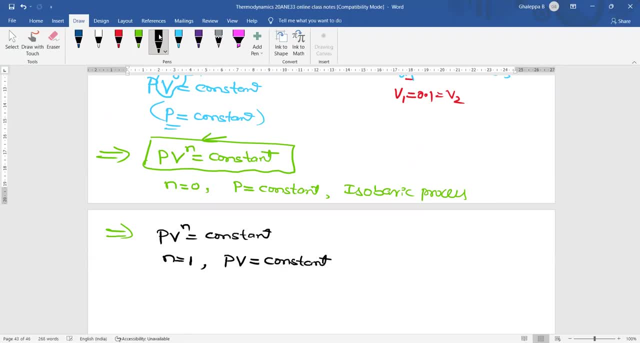 get equation PV is equal to constant. get equation: PV is equal to constant. correct or not, correct or not, correct or not, constant means some value: yeah, constant. constant means some value. yeah, constant. constant means some value. yeah, constant means some value. okay, so this is equal. means some value. okay, so this is equal. 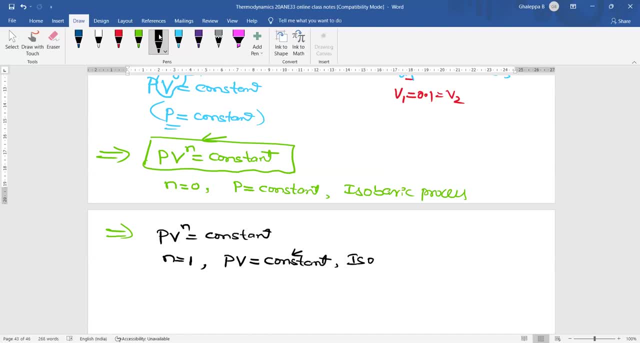 means some value. okay, so this is equal to this. this is equal to means. this is to this. this is equal to means. this is to this. this is equal to means. this is for which process isothermal process? for which process isothermal process? for which process isothermal process? so why I am paying? writing all these? 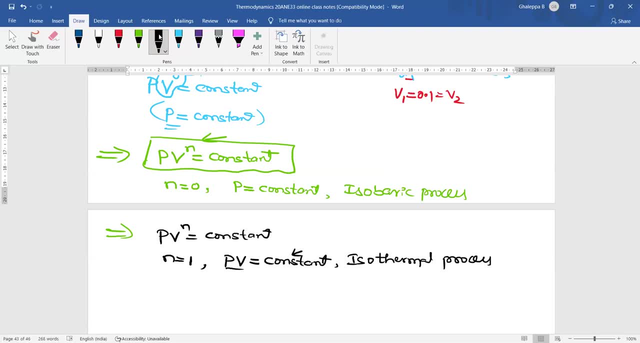 so why I am paying writing all these? so why I am paying writing all these equations? are these equations will be equations? are these equations will be equations? are these equations will be used for numericals? okay in the used for numericals. okay in the used for numericals. okay in the numerical. he will give isothermal. 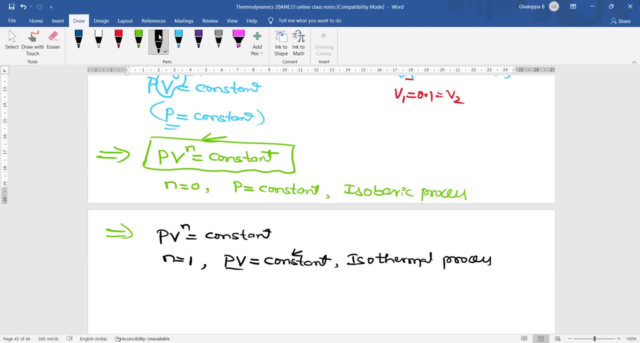 numerical. he will give isothermal numerical, he will give isothermal process. the volume is 0.1 in the process. the volume is 0.1 in the process. the volume is 0.1 in the beginning. volume is 0.5 at the end. 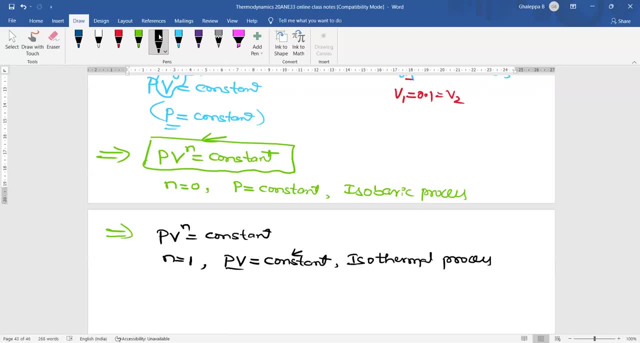 beginning volume is 0.5 at the end. beginning volume is 0.5 at the end. pressure is 1 bar at the beginning. pressure is 1 bar at the beginning. pressure is 1 bar at the beginning. calculate pressure at the end of the. 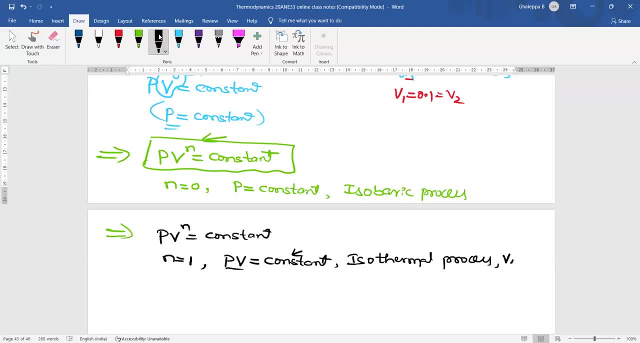 calculate pressure. at the end of the calculate pressure. at the end of the process, you will you v1, you will you v2 process. you will you v1, you will you v2 process. you will you v1, you will you v2, you will you p1, and he may ask you to. 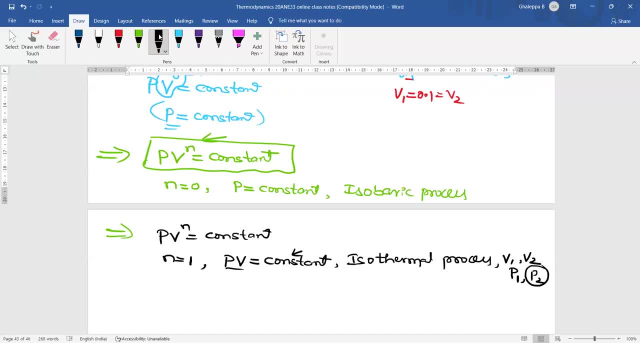 you. will you p1 and he may ask you to you. will you p1 and he may ask you to calculate p2 for isothermal process v1. calculate p2 for isothermal process v1. calculate p2 for isothermal process v1 will be given point 1. v2 will be given. 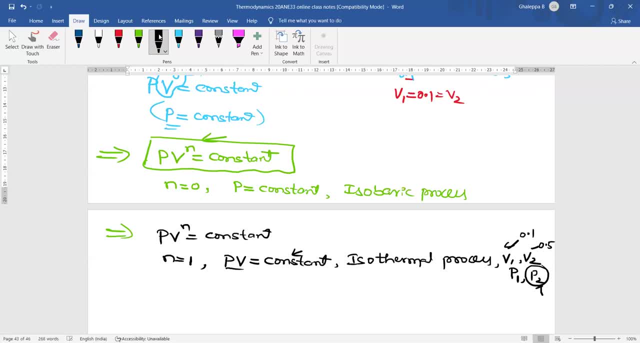 will be given point 1. v2 will be given. will be given point 1. v2 will be given point 5 and he may ask to calculate p2- point 5 and he may ask to calculate p2- point 5 and he may ask to calculate p2 and p1. will be given 2 bar. what will do? 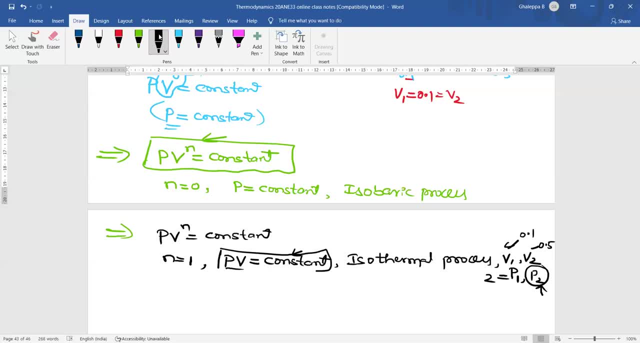 and p1 will be given 2 bar. what will do? and p1 will be given 2 bar. what will do for isothermal? you apply this equation for isothermal. you apply this equation for isothermal. you apply this equation at point number 1: p1- v1 is equal to. 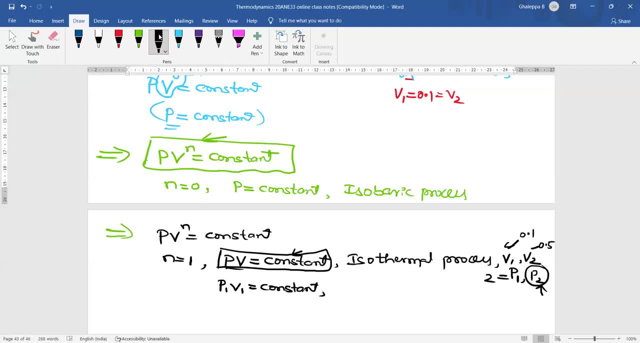 at point number 1, p1- v1 is equal to. at point number 1: p1- v1 is equal to constant. this is at point number 1, same constant. this is at point number 1, same constant. this is at point number 1, same equation. you write at point number 2: 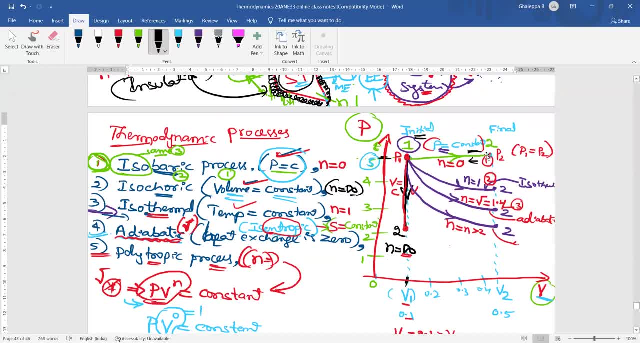 equation: you write at point number 2. equation: you write at point number 2. point number 2 means end of the process. point number 2 means end of the process. point number 2 means end of the process. point number 2 is end of the process. 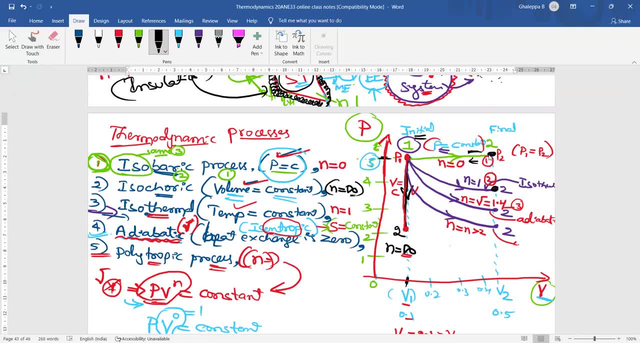 point number 2 is end of the process. point number 2 is end of the process. that is final process. here is a final. that is final process. here is a final. that is final process. here is a final. here is point number 2 is final, end of. 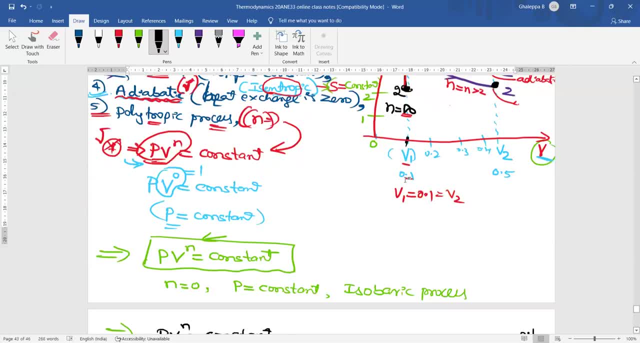 here is point: number 2 is final. end of the process is final. okay, so point the process is final. okay, so point the process is final. okay, so point number 2: I will equation. I will write p. number 2: I will equation. I will write p. 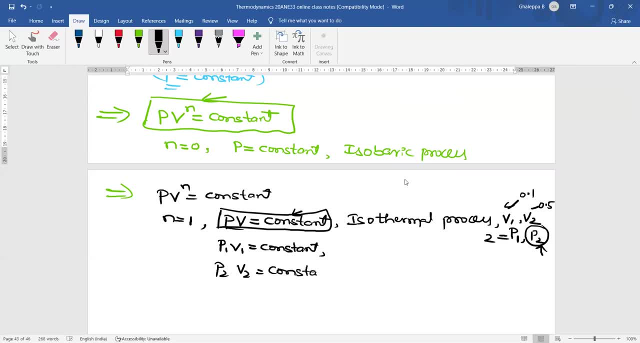 number 2. I will equation. I will write: p 2 v 2 is equal to constant. 2 v 2 is equal to constant. 2 v 2 is equal to constant. so right hand side constant means same. so right hand side constant means same. 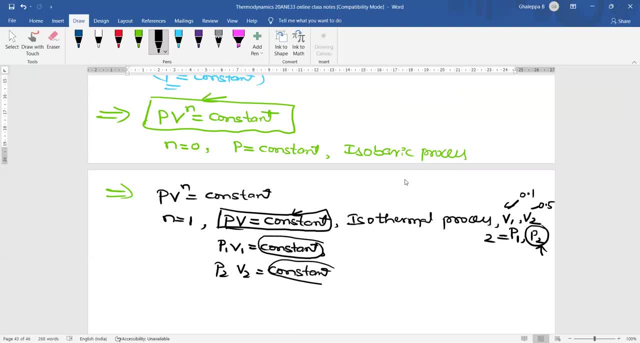 so right hand side, constant means same value. here is also some value. same same value, here is also some value. same same value, here is also some value. same same value is reflecting here: constant right value is reflecting here. constant right value is reflecting here. constant right hand side is same, then obviously left. 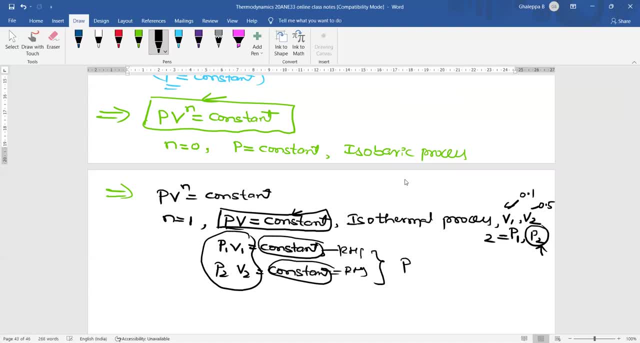 hand side is same, then obviously left hand side is same, then obviously left hand side will be equal to each other. so hand side will be equal to each other, so hand side will be equal to each other. so, based on this, p1- v1 is equal to p2- v2 is. 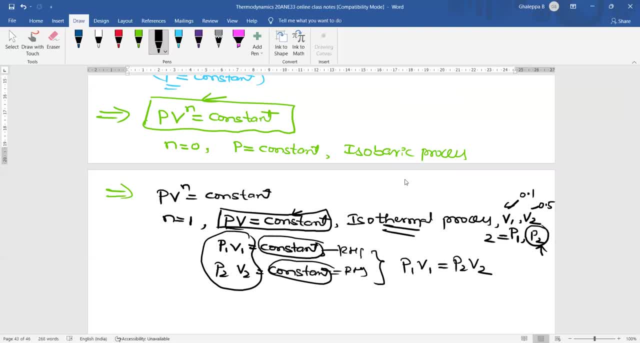 based on this: p1. v1 is equal to p2. v2 is based on this: p1. v1 is equal to p2. v2 is an expression for isothermal. here. v1 is an expression for isothermal. here. v1 is an expression for isothermal. here. v1 is given substitute as 0.1 v2 is given. 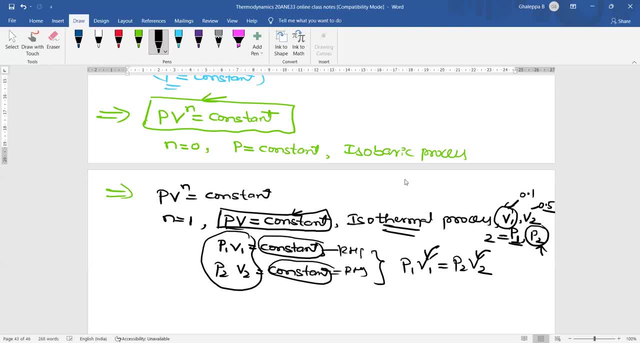 given substitute as 0.1 v2 is given. given substitute as 0.1 v2 is given. substitute as 0.5 p1 is given substitute. substitute as 0.5 p1 is given substitute. substitute as 0.5 p1 is given, substitute as 2 and calculate p2 so to calculate. 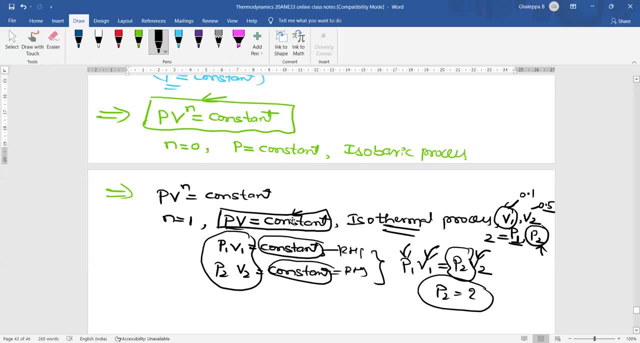 as 2 and calculate p2, so to calculate as 2 and calculate p2, so to calculate, such type of unknowns will be using such type of unknowns will be using such type of unknowns will be using this equation, not only this equation, this equation, not only this equation. 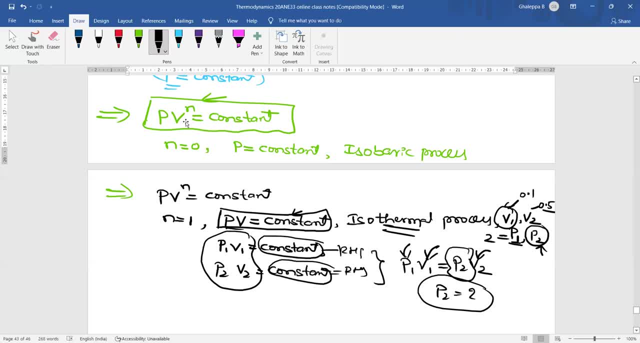 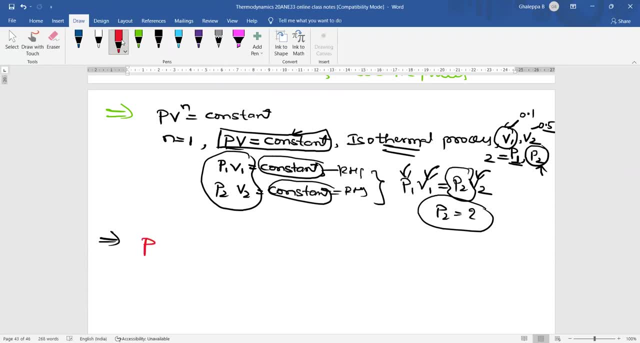 this equation, not only this equation. similarly this equation also. pressure is similarly this equation also. pressure is similarly this equation also. pressure is equal to constant. okay, now I will write equal to constant. okay, now I will write equal to constant. okay, now I will write one more equation: PV to the power of. 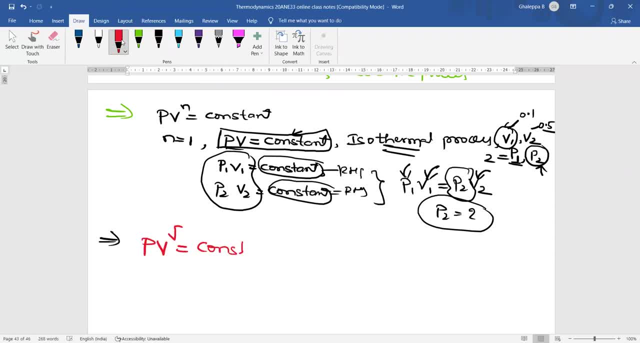 one more equation PV to the power of one more equation PV to the power of gamma is equal to constant. if I write, gamma is equal to constant. if I write, gamma is equal to constant. if I write like this: this is for which process my. like this: this is for which process my 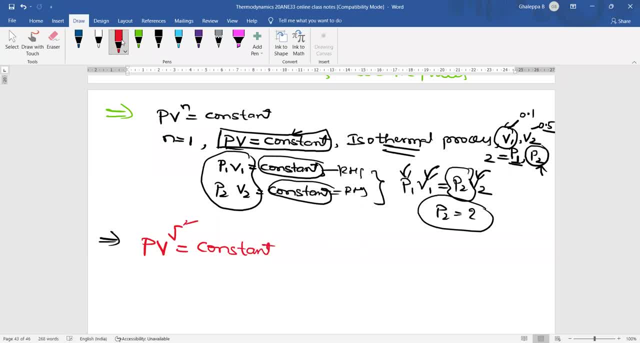 like this: this is for which process my dear strengths whenever I read gamma, dear strengths whenever I read gamma, dear strengths whenever I read gamma. this is for adiabatic adiabatic process. this is for adiabatic adiabatic process. this is for adiabatic adiabatic process, the same. 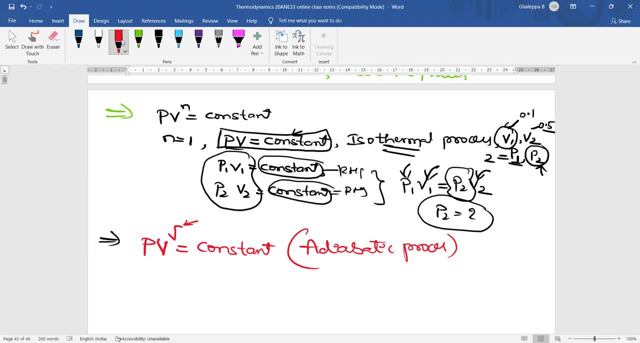 the same, the same same. he may ask you to calculate adiabatic same. he may ask you to calculate adiabatic same. he may ask you to calculate adiabatic index value or pressure. he will index value or pressure. he will index value or pressure. he will give V 1. you will give V 2. he will give P 2. give V 1, you will give V 2, he will give P 2. give V 1, you will give V 2, he will give P 2 and he may ask you to calculate P 1 and he may ask you to calculate P 1. 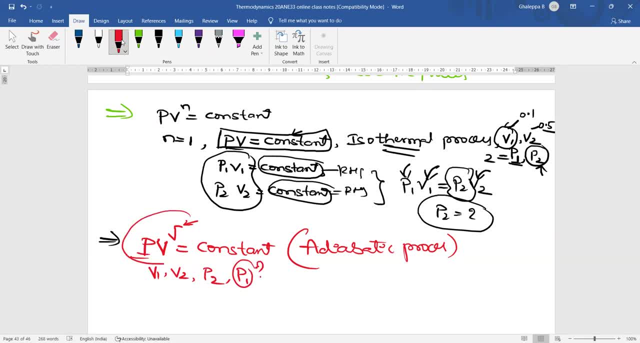 and he may ask you to calculate P 1 in this case. how will you write first you in this case? how will you write first you in this case, how will you write first? you write this equation at point number 1. write this equation at point number 1. 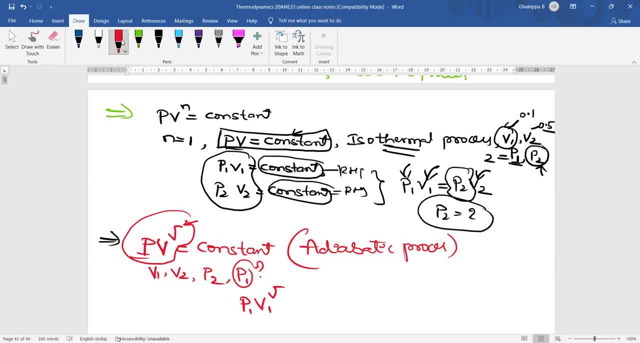 write this equation at point number 1. how will you write P 1 V 1 to the power? how will you write P 1 V 1 to the power? how will you write P 1 V 1 to the power? of gamma is equal to constant. this is at. 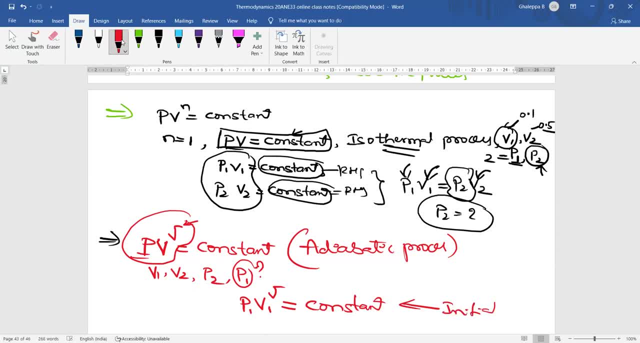 of gamma is equal to constant. this is at: of gamma is equal to constant. this is at first point, initial point. similarly how, first point, initial point. similarly how, first point, initial point. similarly, how to write the second point at the same. to write the second point at the same. 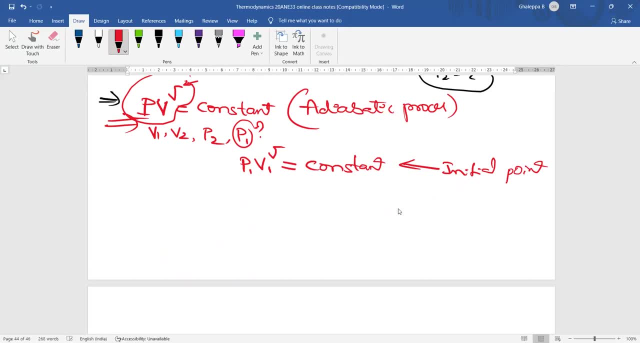 to write the second point at the same equation: adiabatic index equation. equation adiabatic index equation. equation adiabatic index equation. adiabatic process equation at final point. adiabatic process equation at final point. adiabatic process equation at final point. final point is to constant. okay, right. 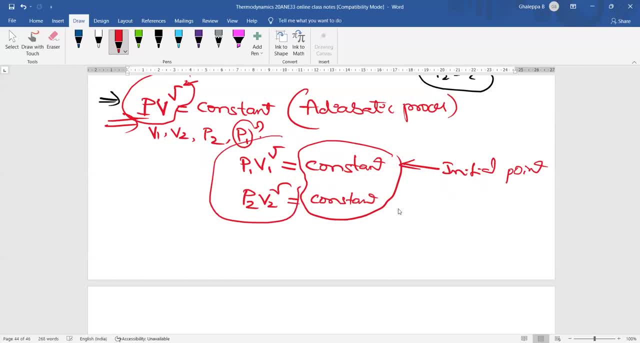 final point is to constant. okay, right, final point is to constant. okay, right hand side is same. obviously, left side hand side is same. obviously, left side hand side is same. obviously, left side, left hand side values will be remain same. left hand side values will be remain same. 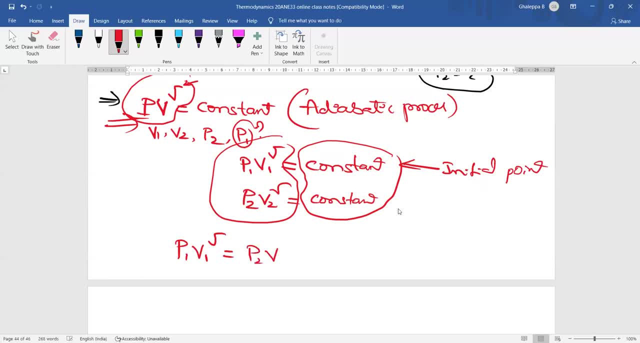 left hand side values will be remain same. so P 1 V 1 to the power of gamma. is so P 1 V 1 to the power of gamma. is so P 1 V 1 to the power of gamma is equal to P 2 V 2 to the power of gamma. 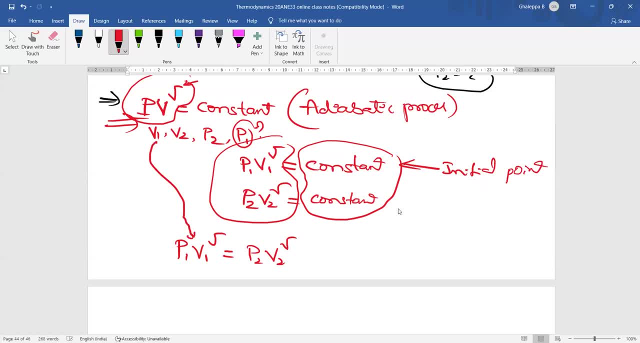 equal to P 2- V 2 to the power of gamma. equal to P 2- V 2 to the power of gamma. here V 1 is given substitute, here V 2. here V 1 is given substitute, here V 2. here V 1 is given substitute. here V 2 substitute. here P 2 is given substitute. 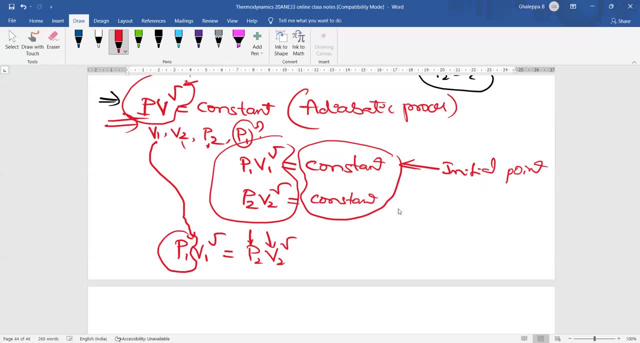 substitute. here P 2 is given substitute. substitute here P 2 is given, substitute here and he is asking P 1. you can here and he is asking P 1. you can here and he is asking P 1. you can calculate P 1 using calculator and one. 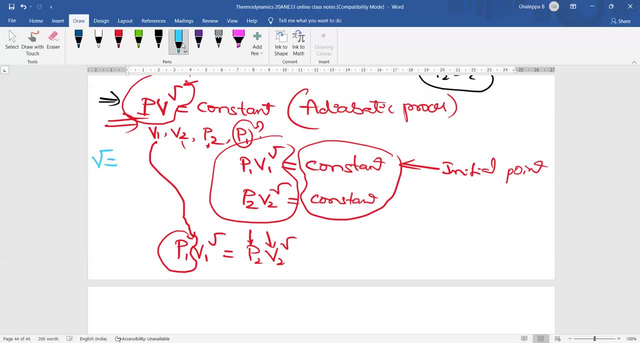 calculate P 1 using calculator and one: calculate P 1 using calculator. and one more point: you always you remember gamma. more point, you always you remember gamma. more point, you always you remember gamma. value is 1.4. this is adiabatic index. value is 1.4. this is adiabatic index. 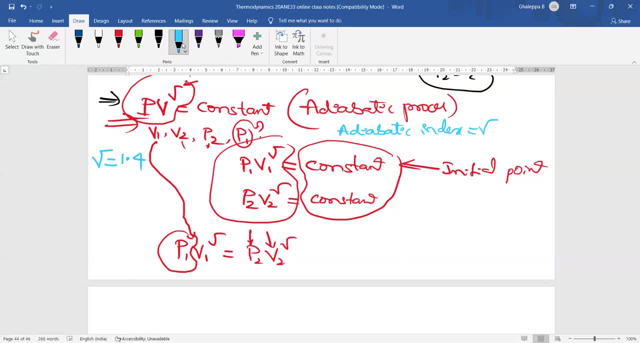 value is 1.4. this is adiabatic index. adiabatic index- that is gamma- is equal to adiabatic index that is gamma, is equal to adiabatic index that is gamma is equal to 1.4. if the this value is given in the 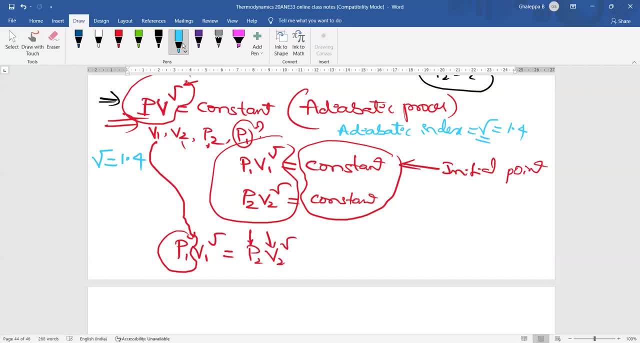 1.4. if the this value is given in the 1.4. if the this value is given in the numerical, use it. otherwise you have to numerical use it, otherwise you have to numerical use it, otherwise you have to remember this value. okay, sometimes he. 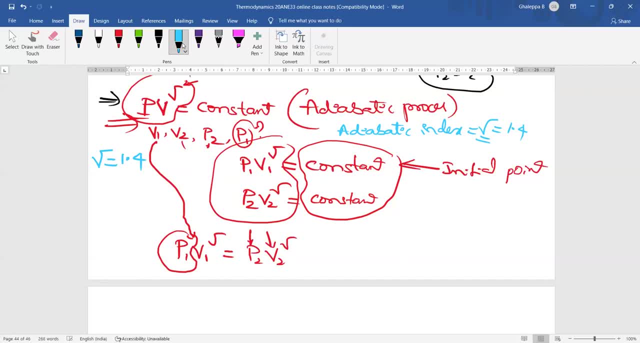 remember this value. okay, sometimes he remember this value. okay, sometimes he may give 1.2- 1.3, but standard values 1.4 may give 1.2- 1.3, but standard values 1.4 may give 1.2- 1.3, but standard values 1.4. understood the last. 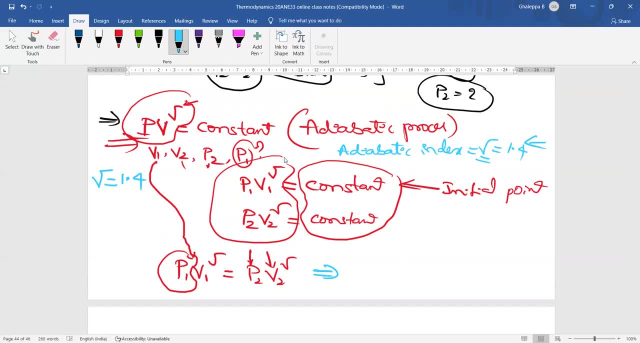 understood the last, understood the last. one more equation is same PV to the one more equation is same PV to the one more equation is same PV to the power of n is equal to constant. what is power of n is equal to constant. what is power of n is equal to constant. what is n? student management here? what is n? 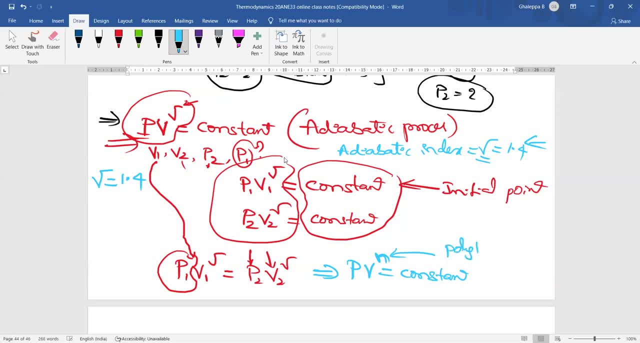 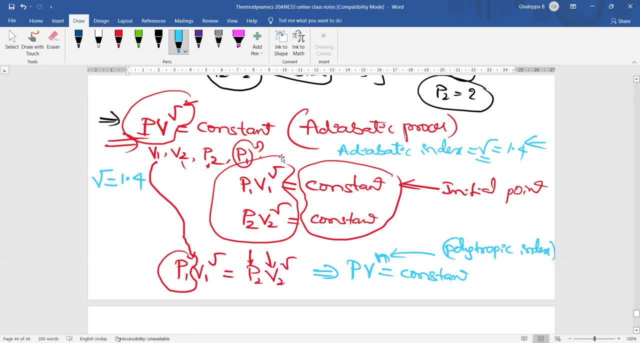 polytropic index. polytropic index. you understood? no, this is little bit you understood. no, this is little bit you understood. no, this is little bit tricky. please watch this video once tricky. please watch this video once tricky. please watch this video once again and you will understand all this. 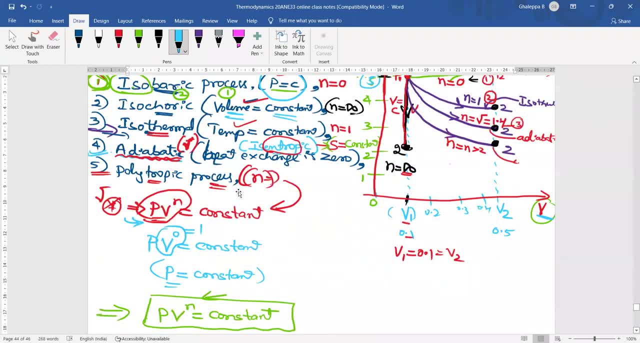 again and you will understand all this again and you will understand all this process. it is very important to solve process. it is very important to solve process. it is very important to solve the numericals first. I request you to the numericals first. I request you to. 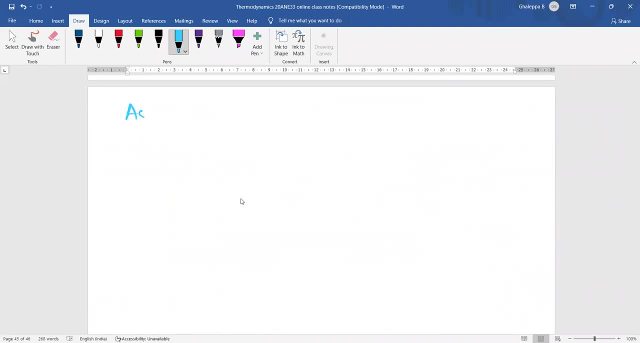 the numericals first. I request you to write the name of the process. what is a? write the name of the process. what is a? write the name of the process. what is a assignment, how you have to this question assignment. how you have to this question assignment. how you have to this question. how they will ask in the question is in. 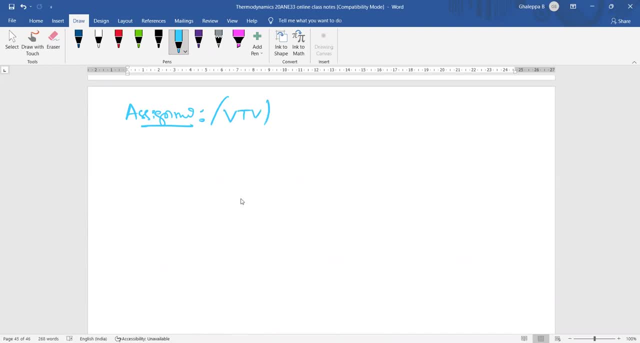 how they will ask in the question is in how they will ask in the question is in the video exam or in the semester exam, the video exam. or in the semester exam, the video exam. or in the semester exam. or in the internal how the question we. or in the internal how the question we. 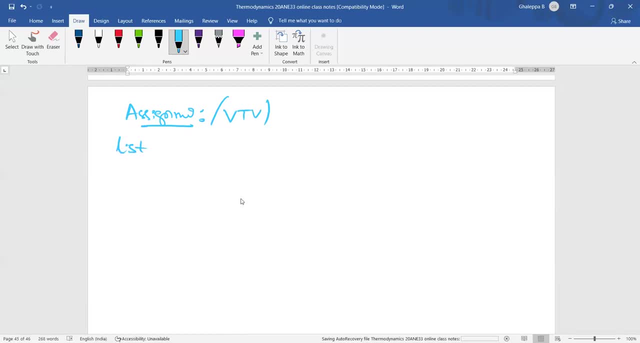 or in the internal, how, the question: we ask least all thermodynamic processes, ask least all thermodynamic processes, ask least all thermodynamic processes. right, the value of n. the right value of right, the value of n. the right value of right. the value of n. the right value of adiabatic index of sorry polytrophic. 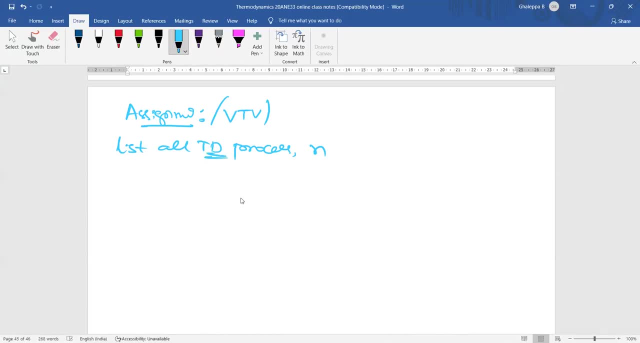 adiabatic index of sorry polytrophic adiabatic index of sorry polytrophic index for all thermodynamic processes. index for all thermodynamic processes. index for all thermodynamic processes. okay, and the same question they may ask. okay, and the same question they may ask. 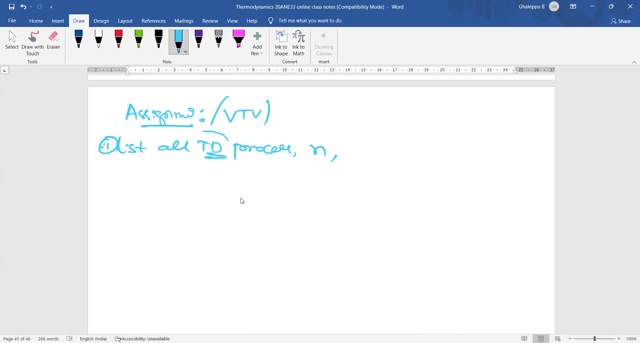 okay, and the same question they may ask: you represent all these thermodynamic. you represent all these thermodynamic. you represent all these thermodynamic process in a single PV diagram, in a process, in a single PV diagram, in a process, in a single PV diagram, in a single PV diagram. this is single PV. 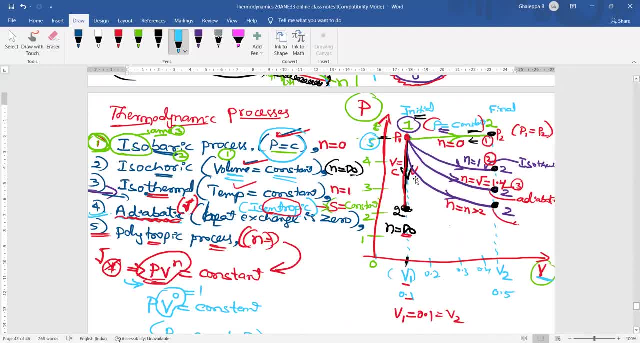 single PV diagram. this is single PV. single PV diagram. this is single PV diagram. why it is called single PV diagram, why it is called single PV diagram, why it is called single PV diagram is all five processes. I have diagram is all five processes. I have diagram is all five processes I have represented in the same PV diagram. if 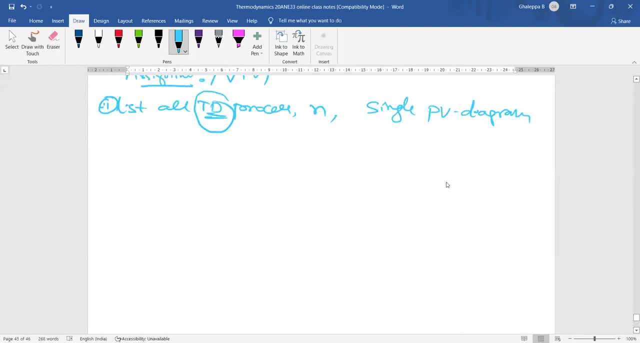 represented in the same PV diagram. if represented in the same PV diagram. if they ask you to drop separately, how they ask you to drop separately, how they ask you to drop separately, how will you drop pressure versus volume? will you drop pressure versus volume? will you drop pressure versus volume? this is for constant pressure, initial. 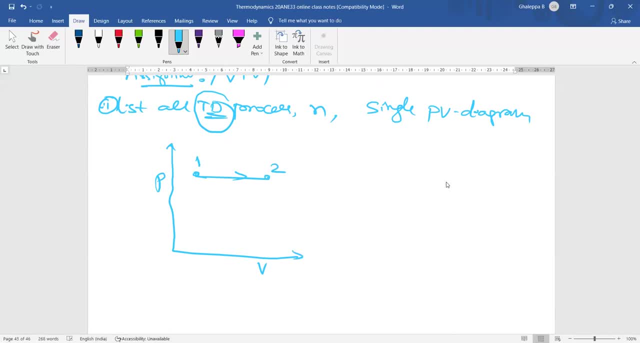 this is for constant pressure, initial. this is for constant pressure initial point, final point, point, final point, point, final point. and for second process: how we need to and for second process, how we need to and for second process, how we need to draw separately PV diagram and PS. 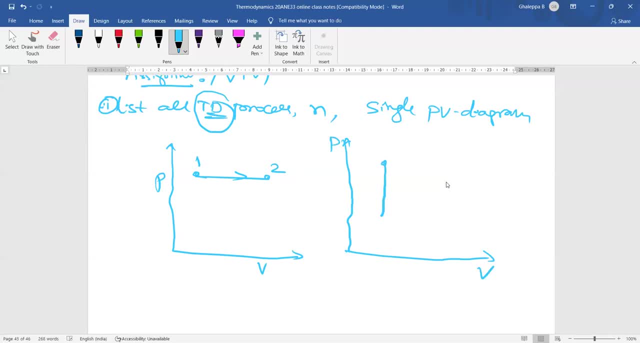 draw separately PV diagram and PS. draw separately PV diagram and PS diagram. PV: this is constant volume diagram. PV: this is constant volume diagram. PV: this is constant volume separately limit, but 90%. they may ask separately limit, but 90%. they may ask separately limit, but 90%. they may ask you to draw the separately rather because 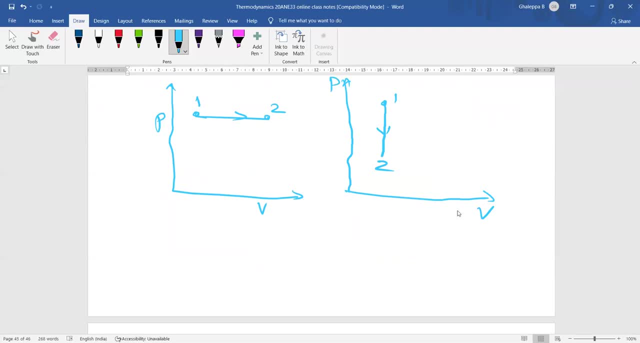 you to draw the separately, rather because you to draw the separately, rather because it is time consuming. they may ask you to. it is time consuming. they may ask you to. it is time consuming. they may ask you to draw all process or represent all process. draw all process or represent all process. 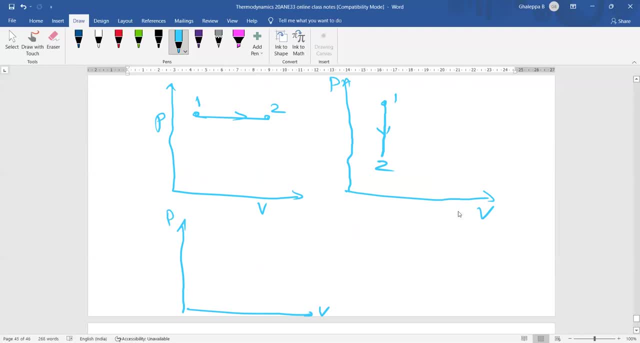 draw all process or represent all process in a single few diagram. single means in a single few diagram. single means in a single few diagram. single means all process. you should draw in the all process. you should draw in the all process. you should draw in the same period area and this is for constant. 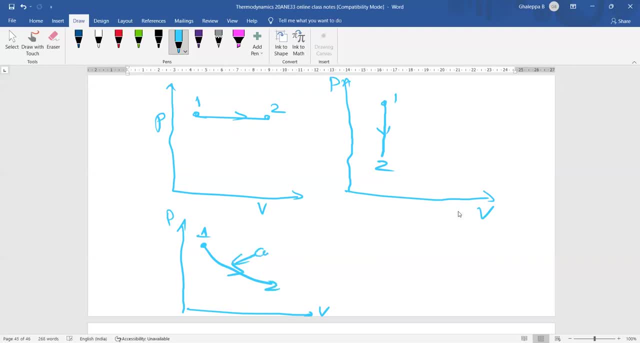 same period area and this is for constant same period area and this is for constant temperature 1 to 2 separately. if you temperature 1 to 2 separately, if you temperature 1 to 2 separately, if you are there, if they ask for separating to. 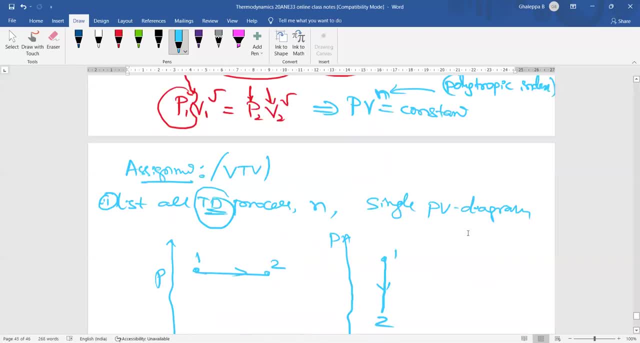 are there if they ask for separating to. are there if they ask for separating to draw like this. otherwise, this is a draw like this. otherwise, this is a draw like this. otherwise, this is a diagram how the question will be asked in. diagram how the question will be asked in. 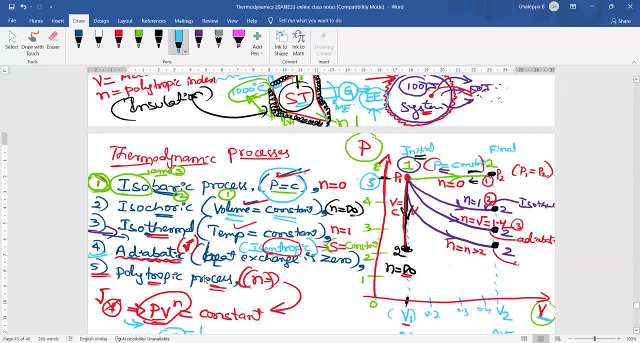 diagram how the question will be asked in the exam: least all thermodynamic, the exam least all thermodynamic, the exam least all thermodynamic processes. and draw the PV diagram for processes and draw the PV diagram for processes and draw the PV diagram for all thermodynamic processes in a single 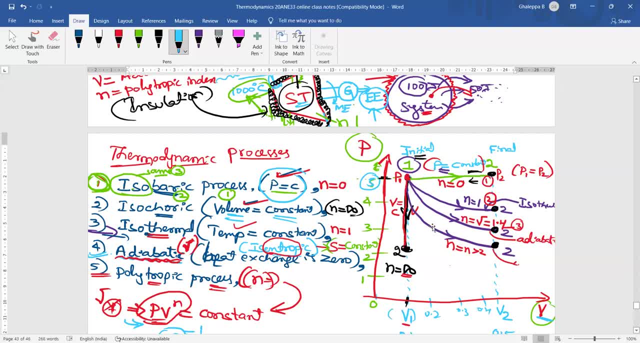 all thermodynamic processes in a single, all thermodynamic processes in a single PV diagram. what is the condition PV diagram? what is the condition PV diagram? what is the condition? condition only condition is consider. condition only condition is consider. condition only condition is consider. initial point is same for all processes. 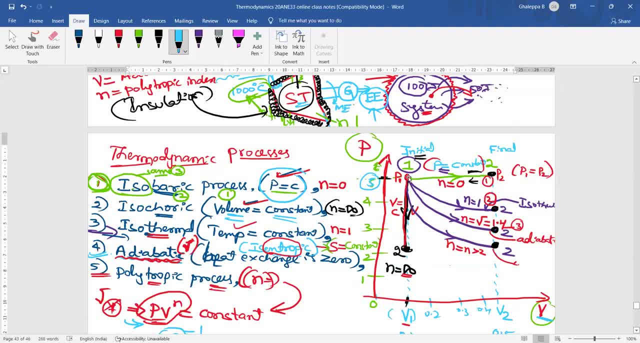 initial point is same for all processes. initial point is same for all processes. look at the PV diagram here, point number. look at the PV diagram here, point number. look at the PV diagram here, point number one is same. I am assuming it is not a. one is same, I am assuming it is not a. 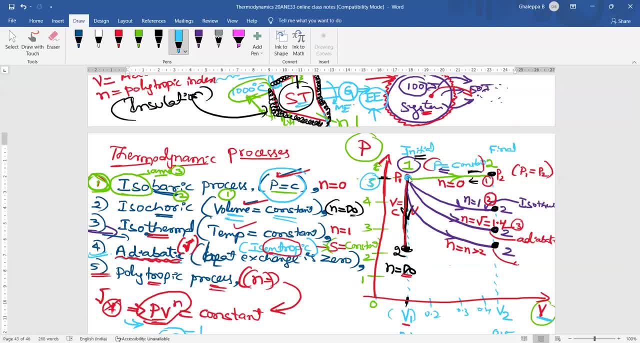 one is same. I am assuming it is not a condition that always it should be same condition that always it should be same condition that always it should be same. I am assuming point number one is initial. I am assuming point number one is initial. I am assuming point number one is initial. point for all the process really point.